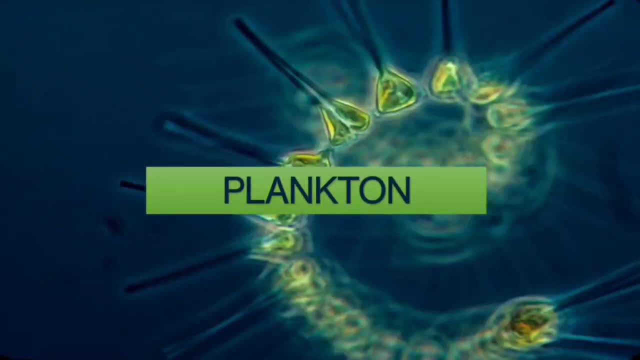 Hi friends, welcome to. To My Knowledge and today we are going to discuss about an important topic for the fisheries and marine biology students and also for UPSC exams, and the topic is plankton. The term plankton is derived from the Greek word for drifter or wanderers. 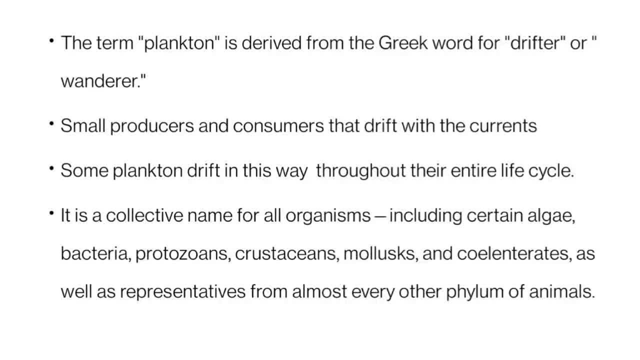 They are small producers and consumers that drift with the water current. The plankton is the productive base of both the marine and freshwater ecosystem, And some plankton drift in this way throughout the entire life cycle, And it is a collective name for all organisms, including serotonin algae, bacteria, protozoan. 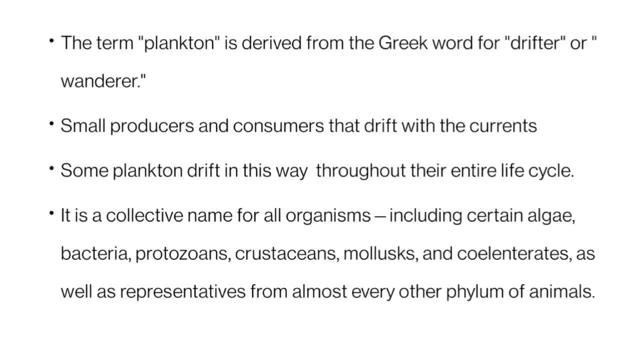 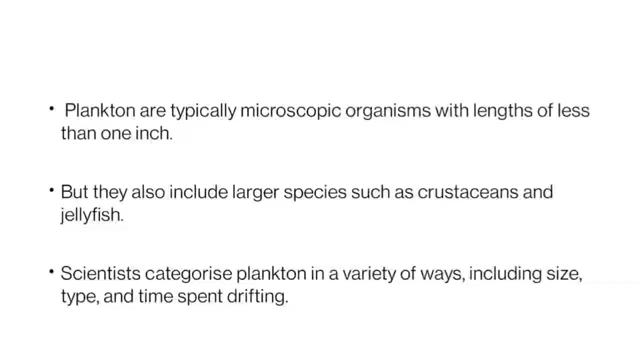 crustaceans, mollusks and sealant rice, as well as a representative from almost every other phylum of animals, And they are non-mortal or too small to swim against the water. current Planktons are typically microscopic organisms with length of less than 1 inch. 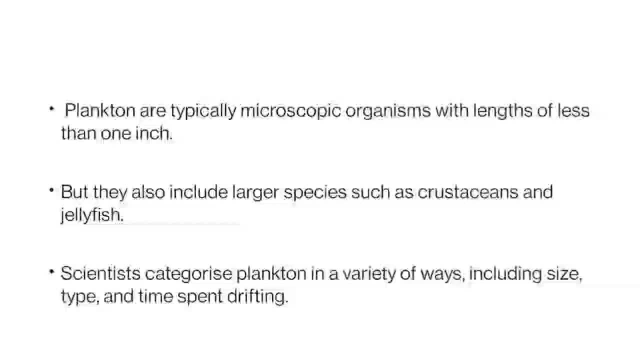 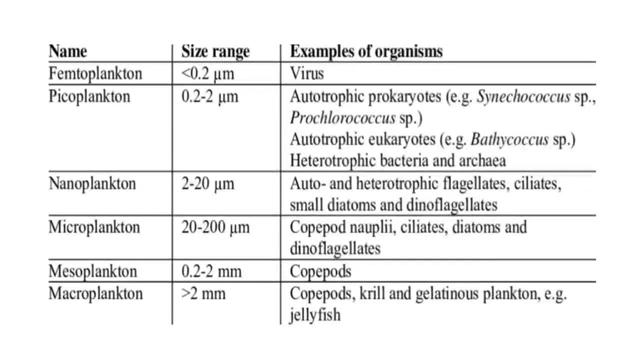 But they also include large species such as crustaceans and jellyfish, And the scientists categorize this plankton In a variety of ways, including on the basis of the size, type and the time spent drifting. On the basis of the size the plankton are classified into. 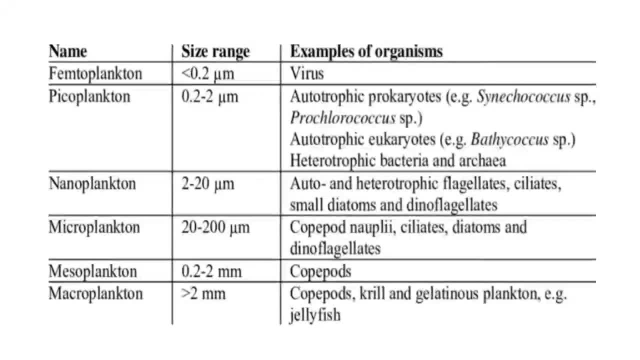 femtoplankton 0.2 micrometer. example virus. picoplankton 0.2 to 2 micrometer. autotropic prokaryotes, autotropic eukaryotes, heterotropic bacteria and aphrodisiacs are examples. 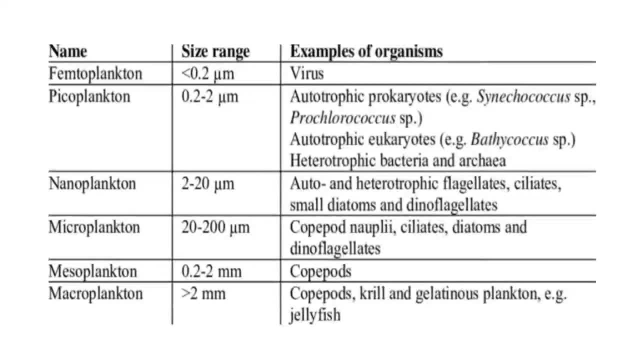 The next one is the nanoplankton 2 to 20 micrometer. They are autotropic and heterotropic. flagellates, ciliates, small diatoms and dinoflagellates. Microplankton 20 to 200 mu m. 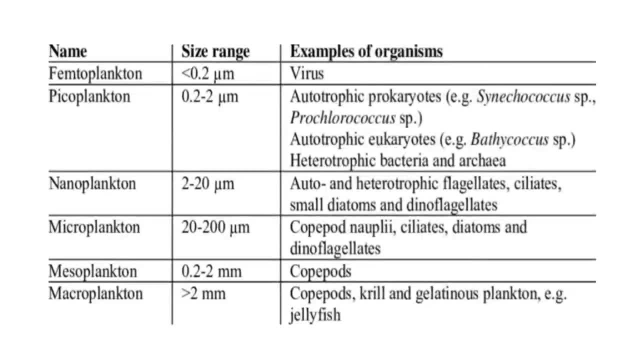 Example: copepodnopoly, ciliates, diatoms and dinoflagellates. Next one is mesoplankton 0.2 to 2 mm. Example copepods. And the last one is the macroplankton which is greater than 2 mm. 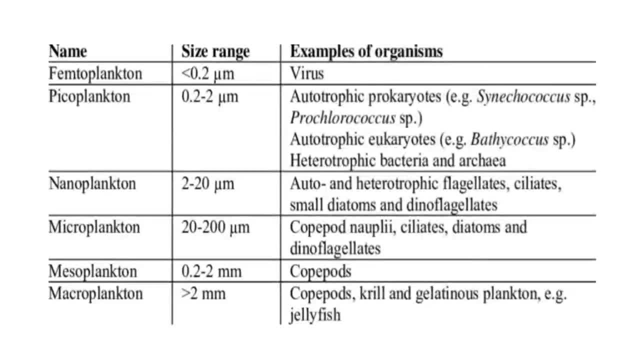 Example: copepodnopoly, ciliates, diatoms and dinoflagellates. Next one is mesoplankton 0.2 to 2 mm. Example copepods. And the last one is the macroplankton which is greater than 2 mm. 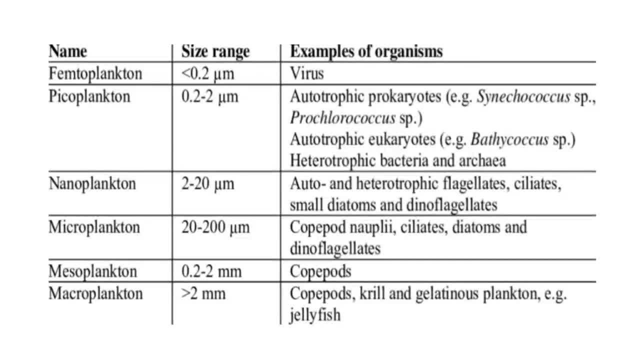 Example: copepod: krill and gelatinous plankton- Example: jellyfish. Try to memorize this table because it is very helpful for your exams and also for further future research. and all And some organisms- Some organisms. Some organisms are classified as plankton when they are young. 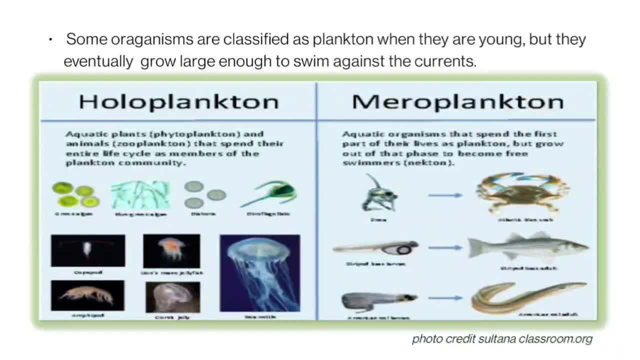 But they are eventually grow larger enough to swim against the water current. And which is the next classification, The plankton is classified on the basis of how much time they spend in the. that organism spend their life in the plankton community. On the basis of that, it is classified into two types. 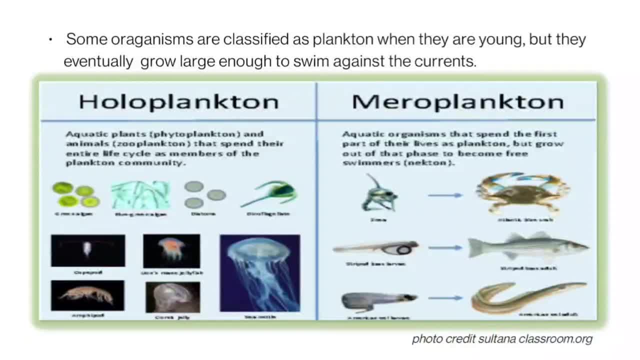 One is holoplankton and the other one is the miroplankton. Holoplankton means if that particular organism spend their entire life cycle as a member of the plankton community. Examples are blue-green algae, diatoms, dinoflagellates, jelly comb jellies, copepods, amphipods, etc. 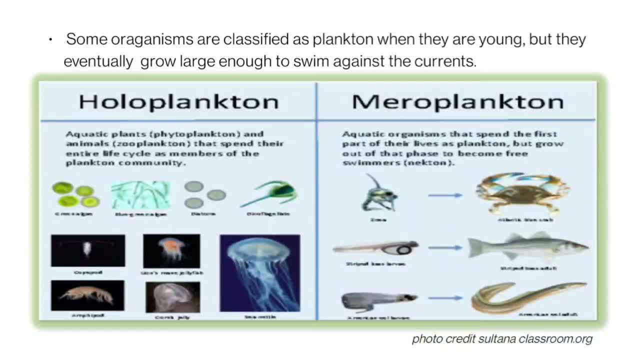 are examples for this: holoplankton And next one is the miroplankton. They are aquatic organisms that spend the first part of their life- means their larval stage- as a plankton And after their growth and they get out of that plankton community as free swimmers. 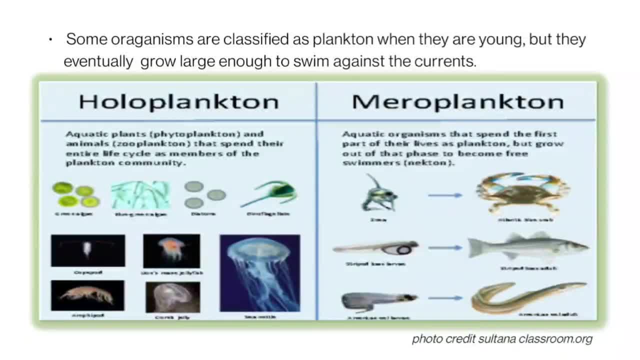 Examples are soya, which is a larvae of the crab, and fish larvae, And when the fish grow up, and after that they left the plankton community, And this is also very important on the basis of the how much time they spend as a organism- spend their life in the plankton community. 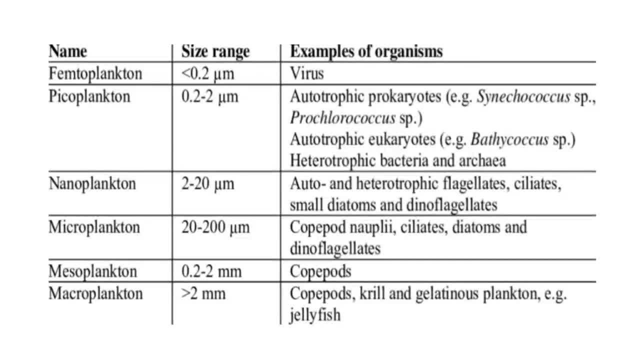 Example: copepod: krill and gelatinous plankton- Example: jellyfish. Try to memorize this table because it is very helpful for your exams and also for further future research. and all And some organisms. Some organisms are classified as plankton when they are young. 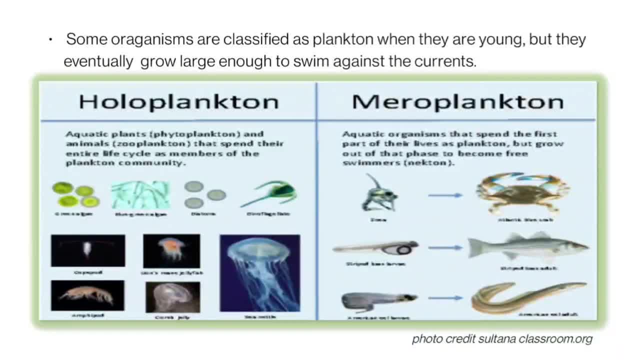 But they are eventually grow larger enough to swim against the water current. And which is the next classification, The plankton is classified on the basis of how much time they spend in the. that organism spend their life in the plankton community. On the basis of that, it is classified into two types. 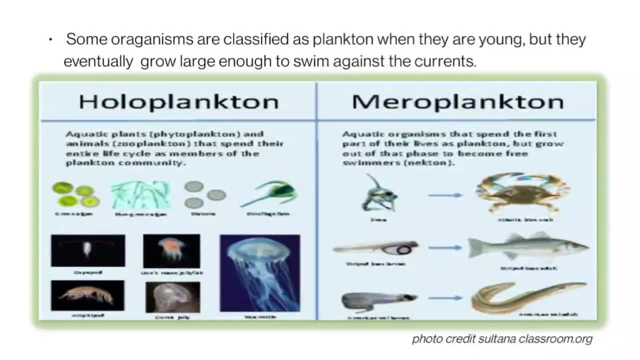 One is holoplankton and the other one is the meroplankton. Holoplankton means if that particular organism spent their spend their entire life cycle as a member of the plankton community. Examples are blue-green algae, diatoms and dinoflagellates. 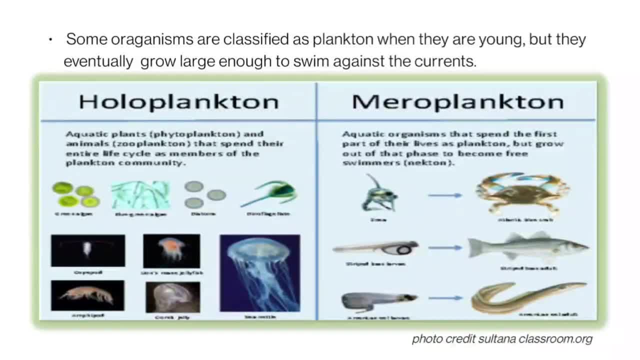 jelly, comb jellies, copepods, amphipods, etc. Examples for this: holoplankton And next one is the meroplankton, Their aquatic organism spend the first part of their life, means their larval stage, as a plankton and after their 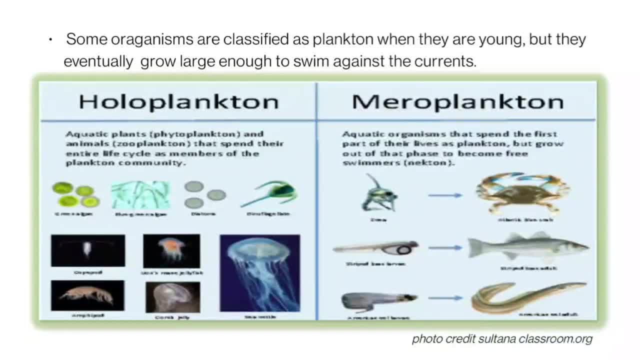 growth and they get out of that plankton community as free swimmers. examples are soya, which is a larvae of the crab, and fish larvae, and when the fish grow up and after that they left the plankton community and this is also very important- on the basis of the 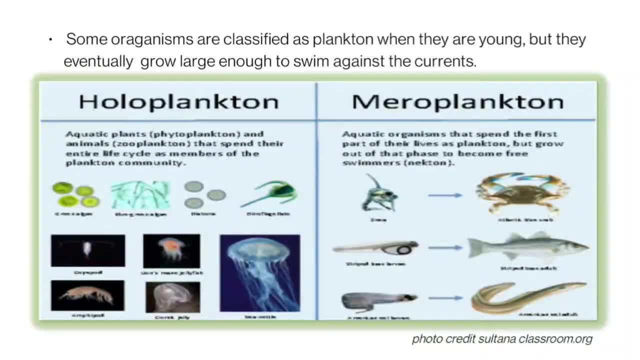 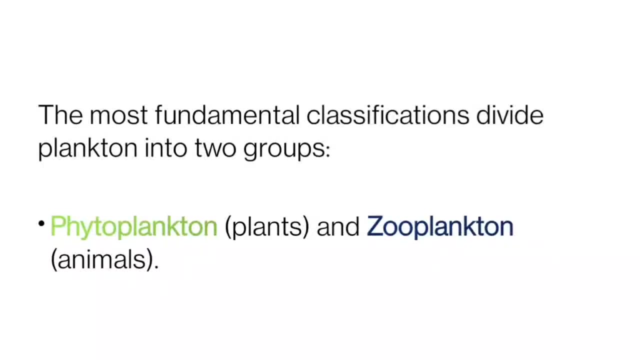 how much time they spend as a organism, spend their life in the plankton plankton community. it's classified into hollow plankton and mirror plankton and this is the most important classification, or the fundamental classification which divide the plankton into two phytoplankton. 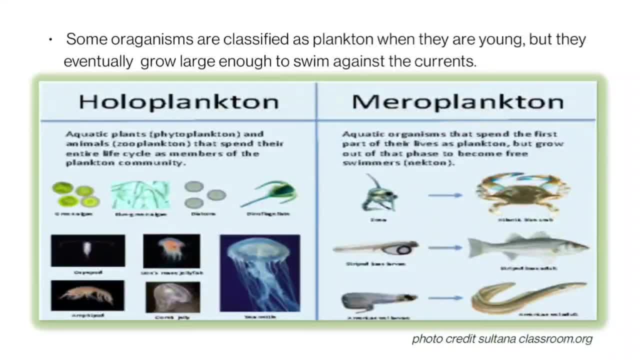 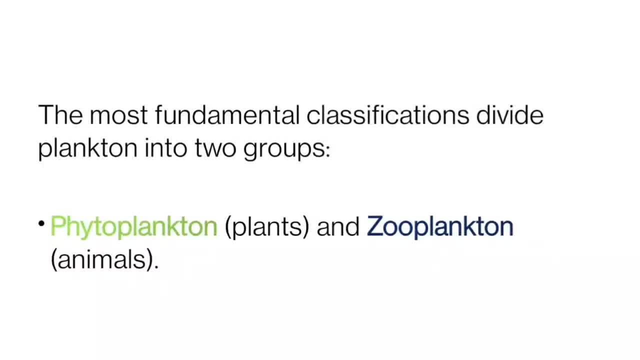 It is classified into holoplankton and miroplankton And this is the most important classification, or the fundamental classification which divide the plankton into two Phytoplankton plants and the zooplankton. they are the animals. 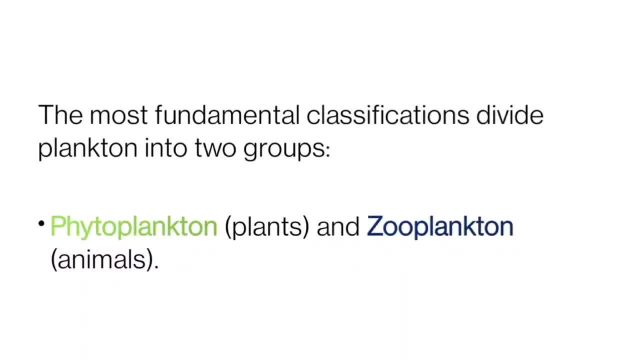 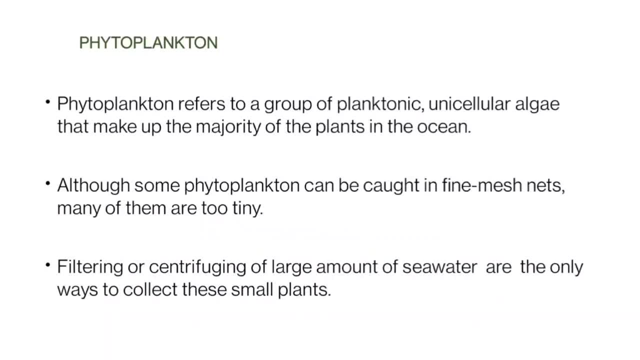 And today only, we are discussing the phytoplankton community and some examples of important phytoplankton groups. The phytoplankton- the phytoplankton produce more than half of the oxygen- yearly oxygen in our planet. The phytoplankton refers to a group of planktonic unicellular algae. 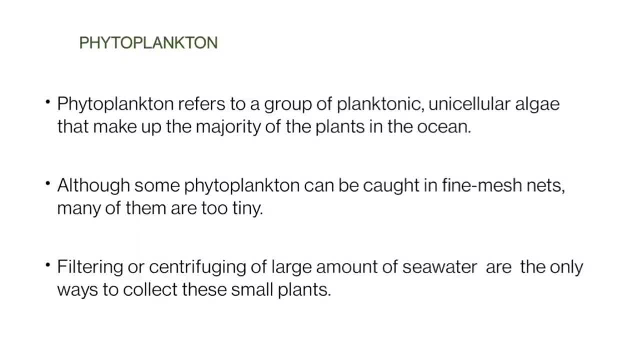 that make up the majority of the plants in the ocean. Although some phytoplankton can be caught in fine mesh nets, and many of them are too tiny, Filtering or centrifuging of large amount of seawater are the only ways to collect these small plants. 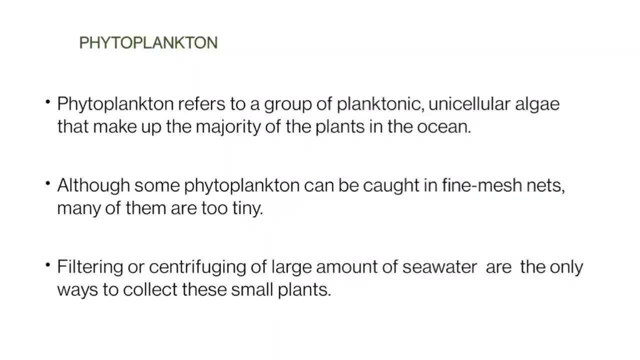 And for the collection or the sampling of this phytoplankton usually use a plankton net with a mesh size of 60 micrometer. And also by another method is by filtering large amount of seawater for centrifuging. And also by another method is by filtering large amount of seawater for centrifuging. 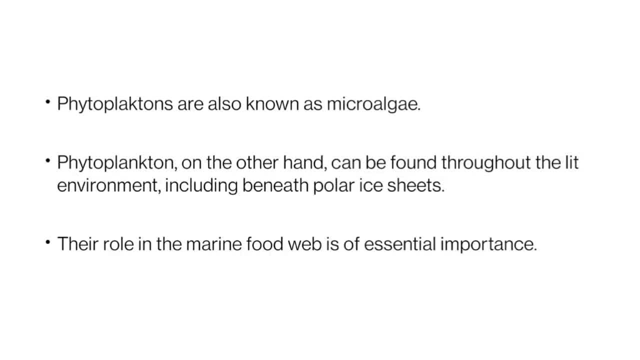 Phytoplankton are also known as microalgae, And the phytoplankton, on the other hand, can be found throughout the lit environment, including beneath the polar ice sheets, And their role in the marine food web is of essential importance. The light intensity of sunlight is an important factor. 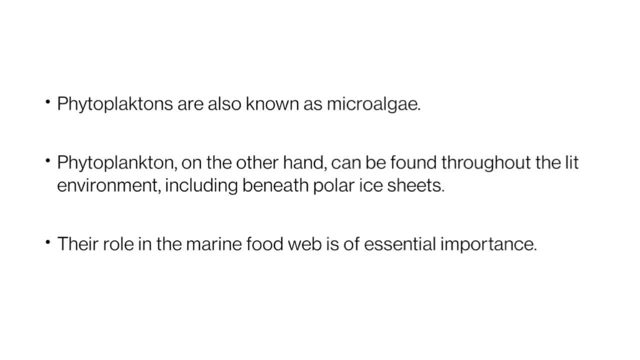 which affects the phytoplankton growth and which is very important. So we are going to discuss them in this video. We are going to discuss them in this video. much helpful for the photosynthesis of this phytoplankton and the nutrient, nutrient availability. 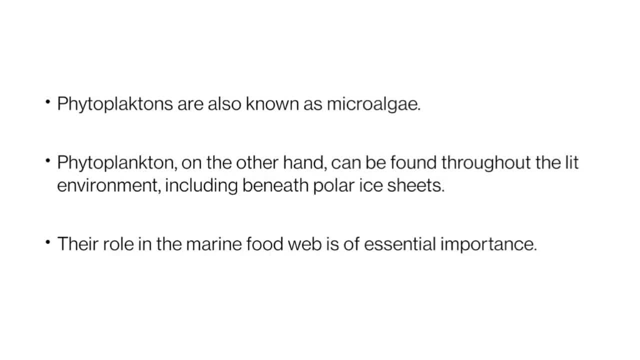 is also important factor for the growth and sustenance of this phytoplankton, and their role in the marine food web is of essential importance because they are the primary producers in the ocean. approximately 5000 species of phytoplankton have been described and new species are continually. 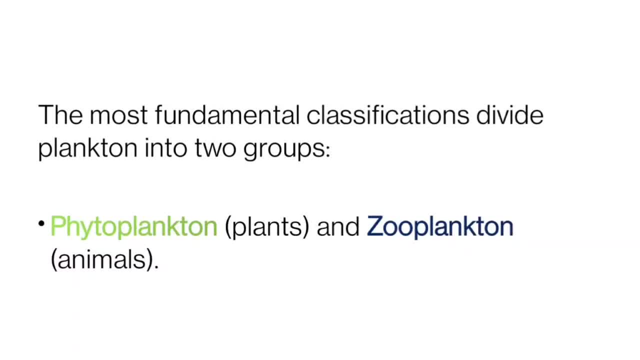 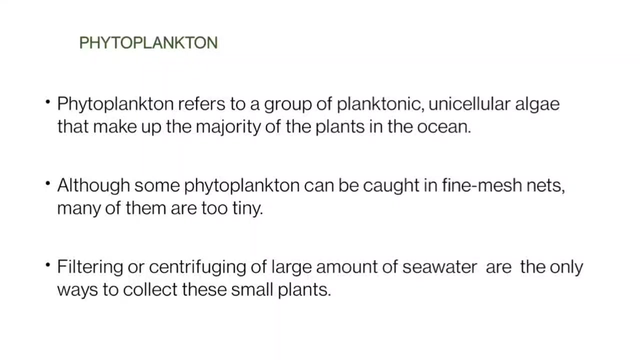 plants and the swimmers plankton. they are the animals and today only we are discussing the phytoplankton community and some examples of important phytoplankton groups. the phytoplankton- the phytoplankton produce more than half of the oxygen yearly oxygen in our planet. the phytoplankton refers to a group. 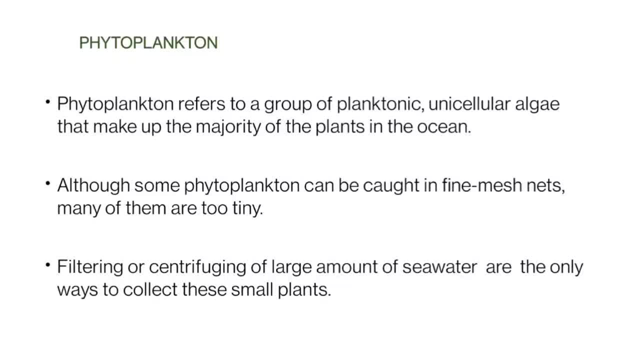 of planktonic unicellular algae that make up the majority of the plants in the ocean. although some phytoplankton can be caught in fine mesh nets, and many of them are too tiny, filtering or centrifuging of large amount of seawater are the only ways to collect these small. 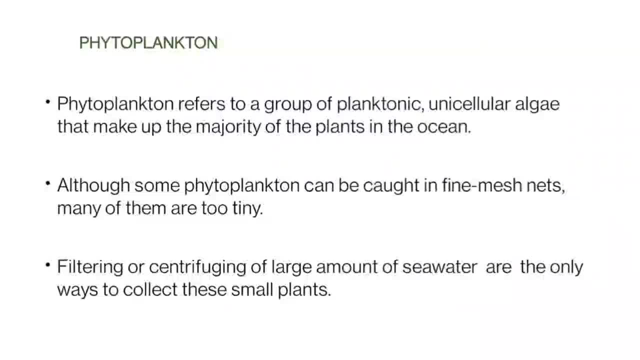 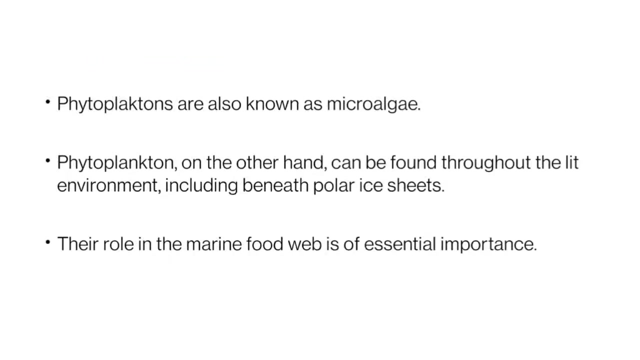 plants, and for the collection or the sampling of this phytoplankton usually use a plankton net with a mesh size of six, sixty micrometer, and also by, and. another method is by filtering large amount of sea sea water for centrifuging. phytoplanktons are also known as micro algae. the phytoplankton, on the other hand, can be 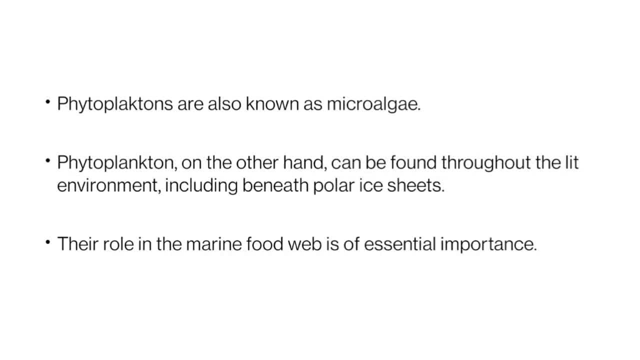 found throughout the lit environment, including beneath the polar ice sheets, and their role in the marine food web is of essential importance. the light intensity, or the sunlight, is an important factor which affected the phytoplankton growth and which is very much helpful for the photosynthesis of this phytoplankton and the 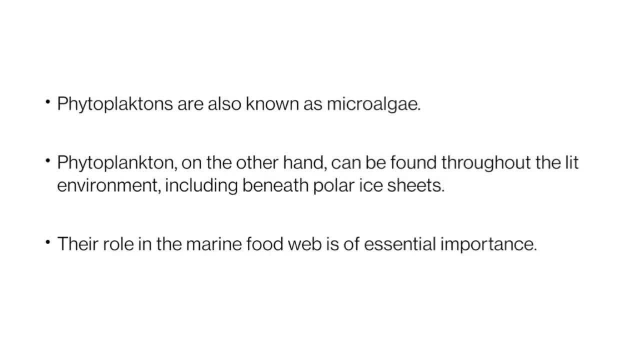 nutrient. nutrient availability is also a important factor for the growth and sustenance of this phytoplankton, and their role in the marine food web is of essential importance because they are the primary producers in the ocean. approximately 5 000 species of phytoplankton have been described, and new species are continually. 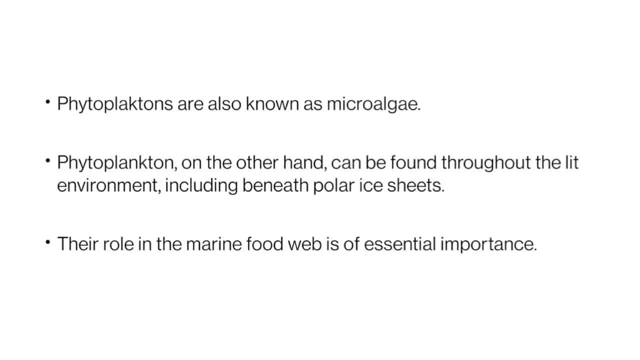 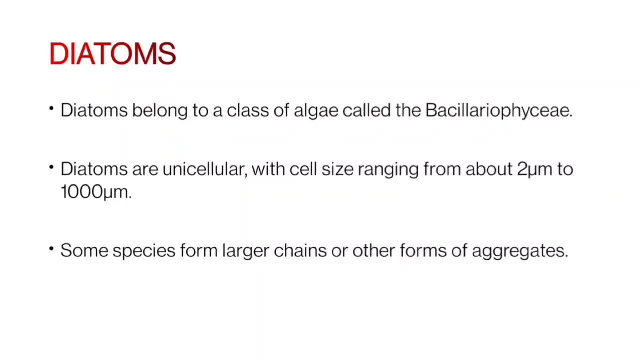 being added to this total. but, and here only, we are discussing about some important groups. the first one is a diatoms. diatoms belong to a class of algae called the bacilliriophysaea. the diatoms are unicellular, with cell size ranging from 5 to 10 percent of the body weight of the 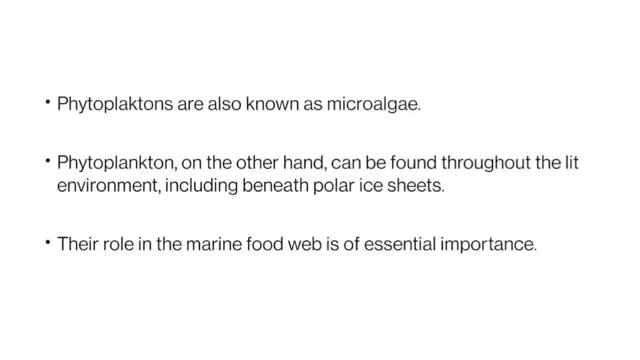 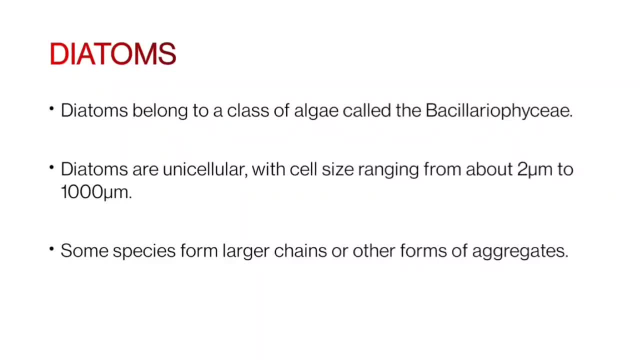 being added to this total. but- and here only- we are discussing about some important groups. the first one is a diatoms. diatoms belong to a class of algae called the bacilliriophysae. the diatoms are unicellular, with cell size ranging from about two micrometer to thousand micrometer, and some species form larger chains or others form 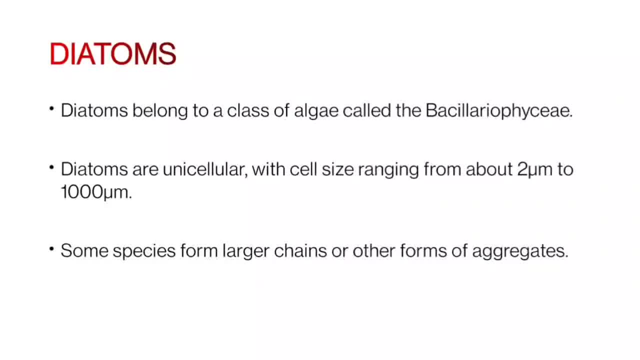 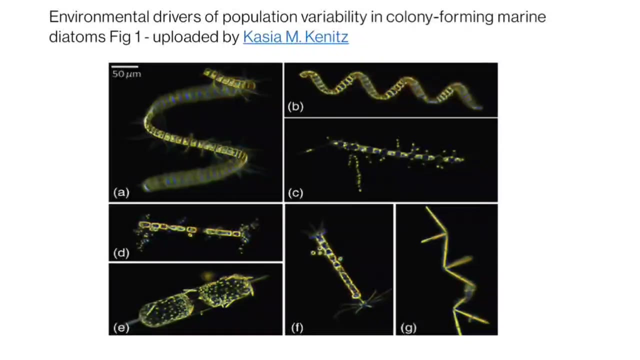 aggregate. there are some chain forming diatoms and also aggregate or mass forming diatoms, and these are some examples- and this is an image i took from the, a publication environmental drivers of population variability in colony forming marine diatoms and in this picture, from a to d? uh, it's the ketos ketoceros species. 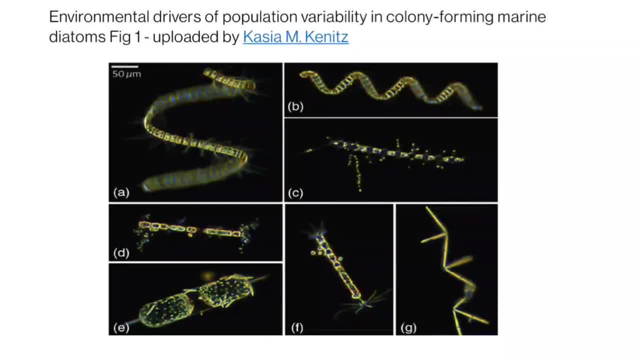 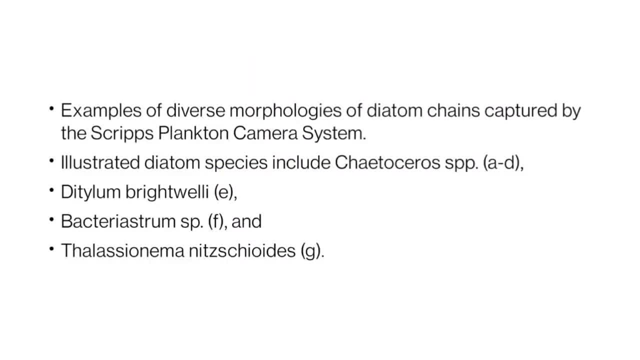 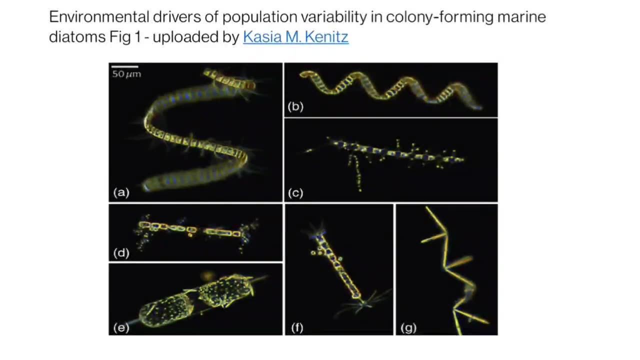 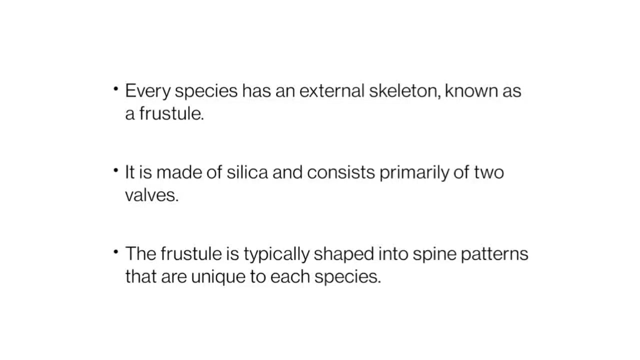 and e is detail and bright valley species and f is the bacteria from species. and the last one is the thalassonyma. g is thalassonyma species and one specialty of this diatom is the. each and every species has an external skeleton which is 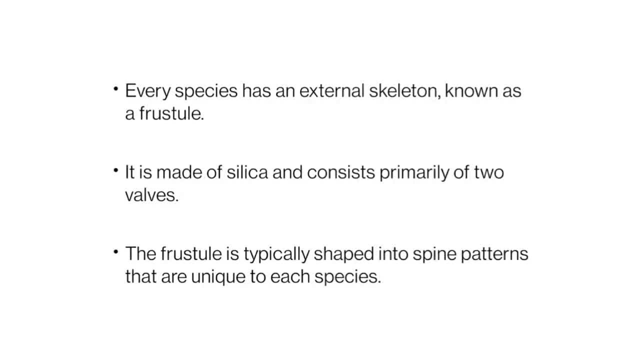 known as the frustules, and these diatoms are actually looked like armored, or shell, like shell, like what you call, which is made up of silica, and this frustule is made up of silica. more¡¡¡¡¡¡¡¡¡¡¡¡¡¡¡¡¡¡¡¡¡¡¡¡¡¡¡¡¡¡¡¡¡¡¡¡¡¡¡¡¡¡¡¡¡¡¡¡¡¡¡¡¡¡¡¡¡¡¿¡¡¡¡¡¡¡¡¡¡¡, ¿¡¡¡¡¡¡¡¡¡¡¡¡¡¡¡¡¡¡¡. 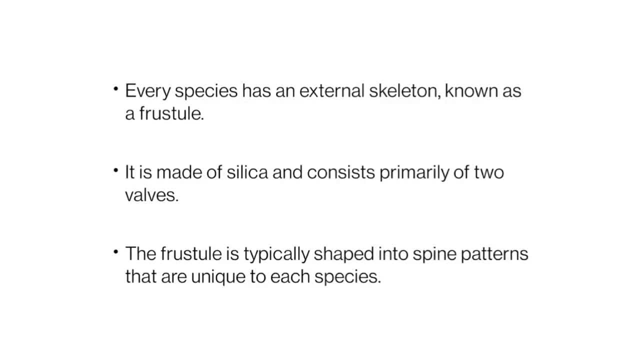 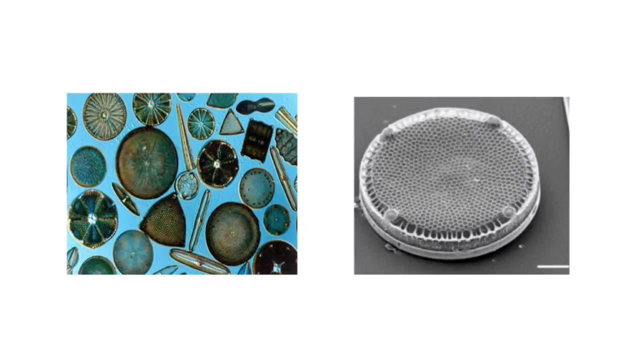 the frustule is typically shaped into spine texteless spine pattern that are unique organizations and the atoms is very diverse and this spine like structure is actually very unique for each species. this is awkward. and the right side, which is a same image of uh casino discus and the astro. right side by the astro plant package are called positionuz巧o co高. there also have kid animal image, ofution or not, plane of local capitalism metal. but in the rest of the project, discussing co reason, now we will discuss the galacticieved we meal s. 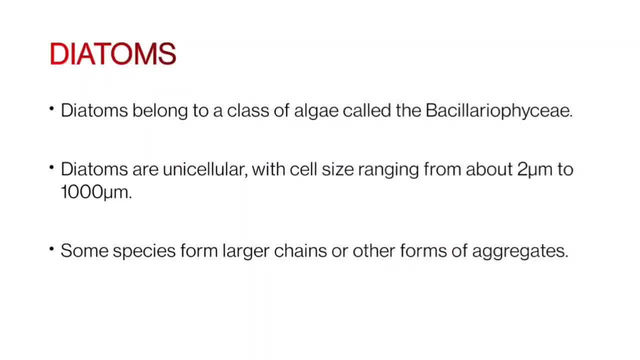 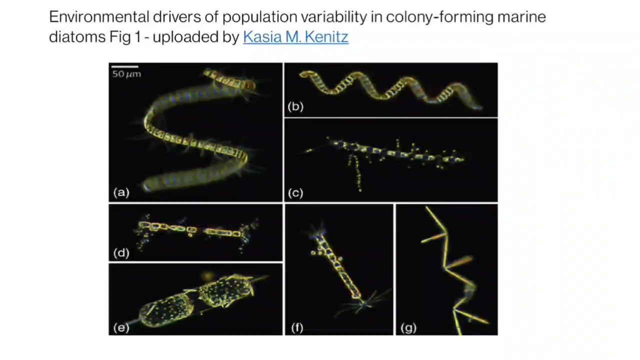 size ranging from about 2 micrometer to 1000 micrometer, and some species form larger chains or others form aggregate. there are some chain forming diatoms and also aggregate or mass forming diatoms, and these are some examples and this is an image i took from the a publication environment. 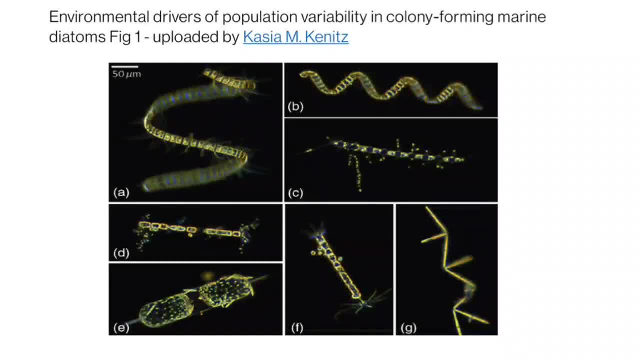 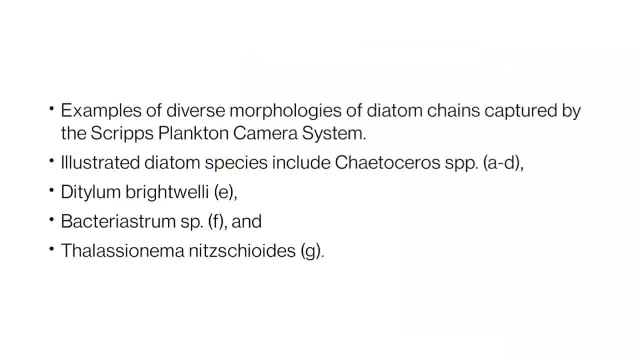 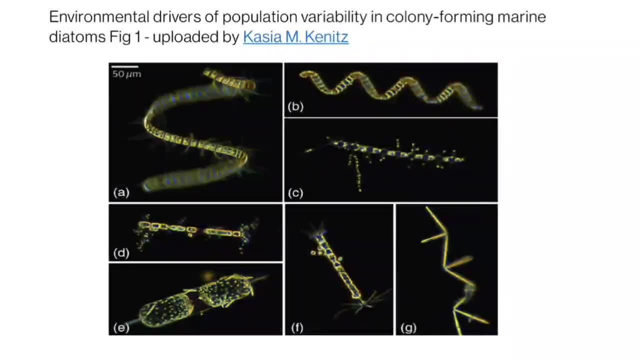 and this is an image i took from the, a publication environment drivers of population variability in colony, forming marine diatoms. and in this picture, from a to d uh, it's the ketos ketoceros species- and he is a detail- and bright valley species, and f is the bacteria from species and the last one is the. 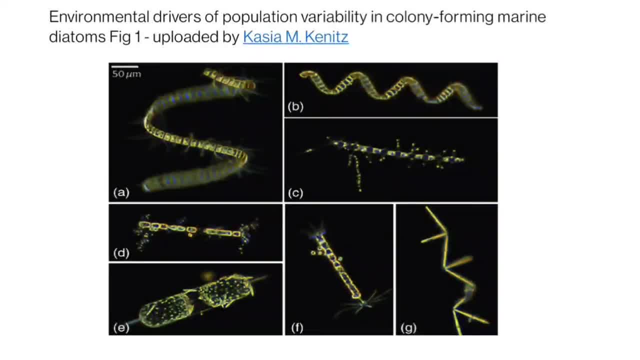 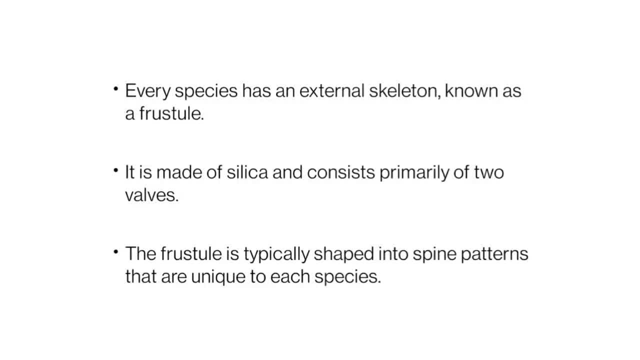 thalassonyma g is thalassonyma species, and one specialty of this diatom is the. each and every species has an external skeleton, which is known as the frustules, and these diatoms are actually looked like armored shell, like shell, like what you call, which is made up of silicon, and this frustule is made up of. 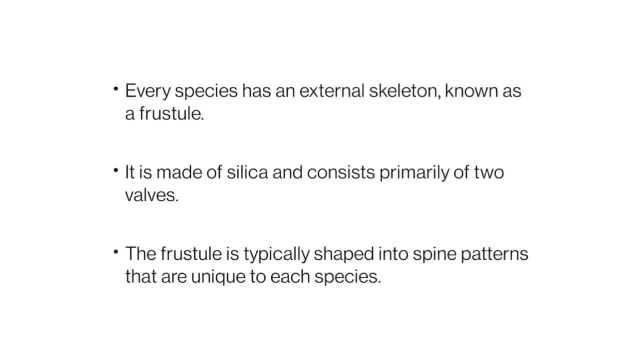 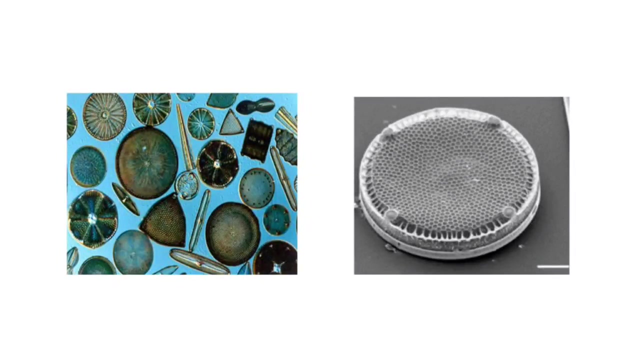 silicon. the frustule is typically shaped into spine pattern that are unique to each species and the diatoms is very diverse and this spine like structure is actually very unique for each species. this is the image of diatoms and the right side, which is a same image of. 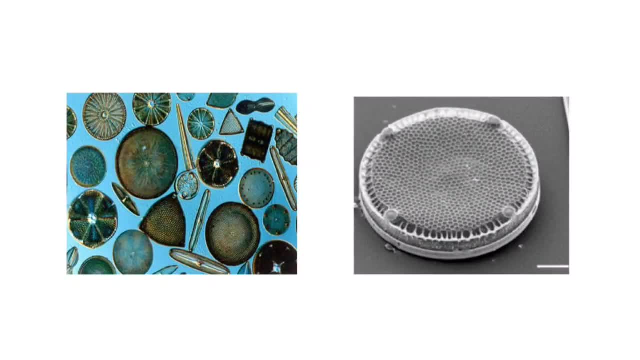 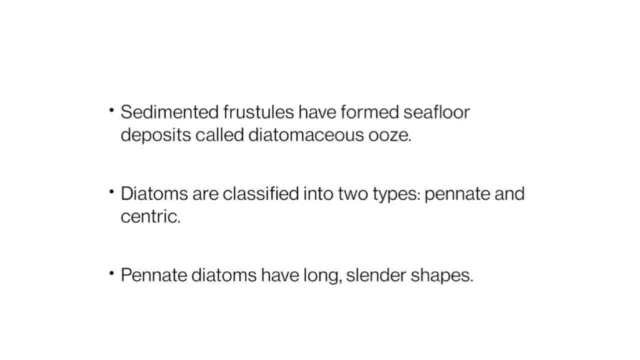 cocinodiscus and the frustule of this cocinodiscus and you can see that spines and all the sedimented frustules have formed seafloor deposits called the diatomaceous oozes. after the death of this, this diatom, these frustules are deposited into the sea bottom. 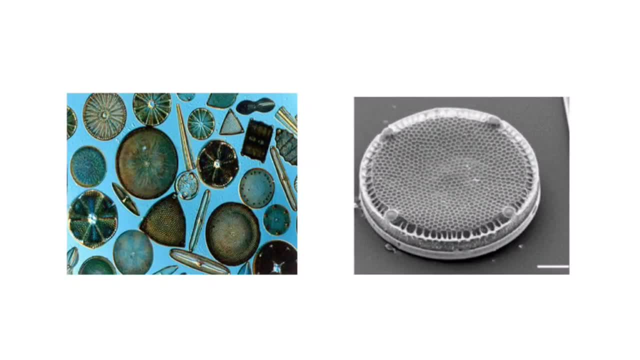 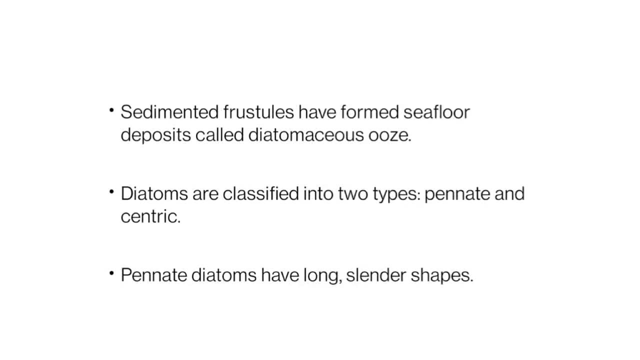 coccinodiscus and the frustule of this coccinodiscus and you can see that spines and all the sedimented frustules have formed seafloor deposits, called the diatomaceous oozes. after the death of this, this diatom, these frustules are deposited into the sea bottom. 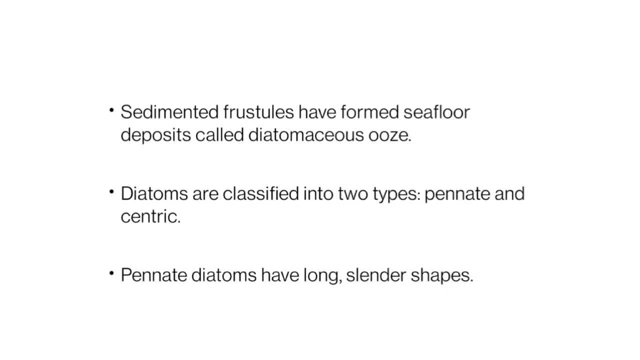 and, as a result, diatomaceous ooze, which is siliceous ooze because the frustule is made up of silica and, as a result, the deposited frustules will result in the formation of siliceous ooze, and the diatoms are classified into two types on the basis of the shape. 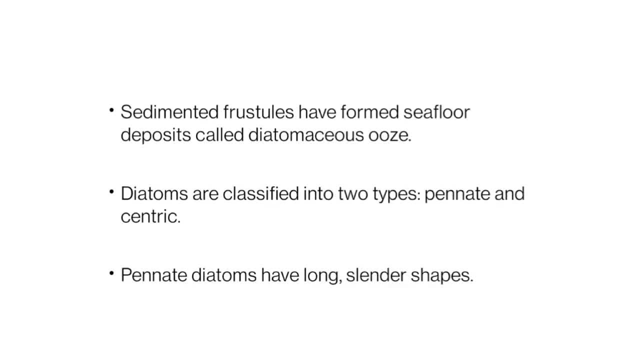 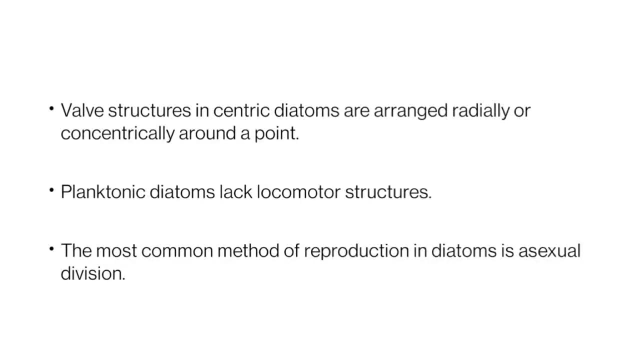 one is the pinnate diatom and the other one is the centric diatom. the pinnate diatom is: these diatoms have an elongated shape. so, and in centric diatoms, the centric diatoms have valves that are arranged radially or concentrically around a point. 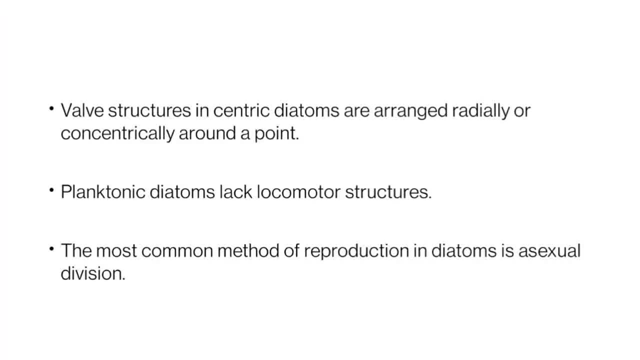 and the most common method of reproduction in diatom is asexual division and in diatoms the method of reproduction is asexual division. and sexual division is also present when diatom is formed, ie this professional Колiplos diatom is made up of diatom that reaches a certain 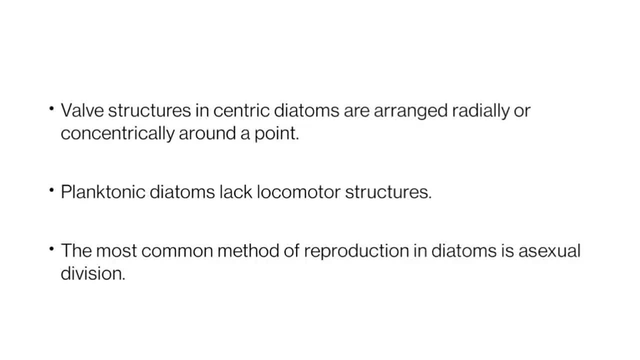 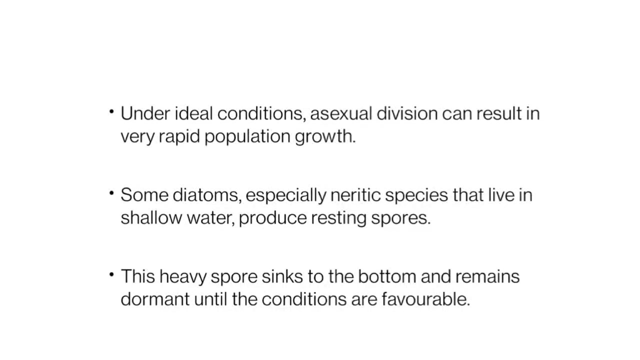 critical minimal size. it undergoes sexual reproduction also, and this as because of this asexual reproduction and which results in the very rapid population growth under optimal conditions, and some diatoms, especially neuritic species that live in shallow water, produce small ruptured 실신. shallow water produce the rusting, rusting spores and this and this heavy 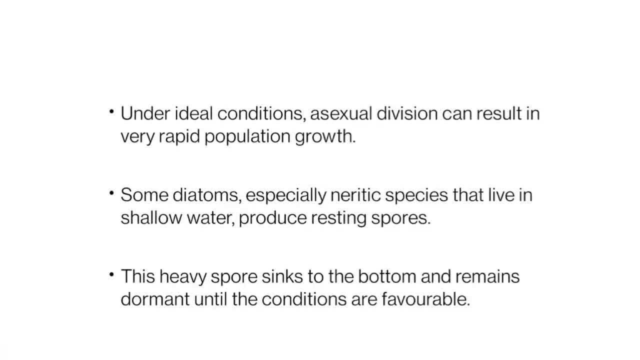 spores actually sink into the bottom and remain dormant until until favorable situations and during unfavorable condition, this diatoms produce rusting spores and when a favorable condition came, and did, will and it will produce and normal planktonic cells over the or these spores transformed into a normal 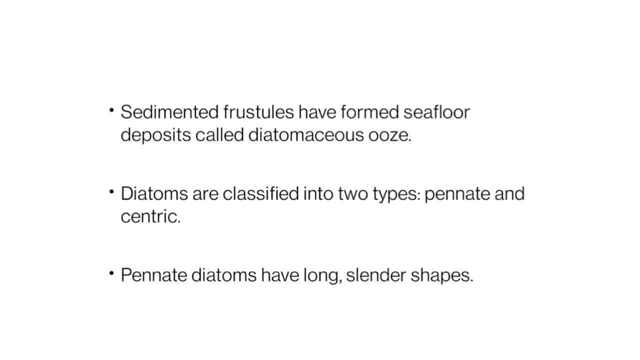 and, as a result, diatomaceous ooze, which is a siliceous ooze because the frustule is made up of silica and, as a result, the deposited frustules will results in the formation of siliceous ooze, and the diatoms are classified into two types on the basis of the shape. 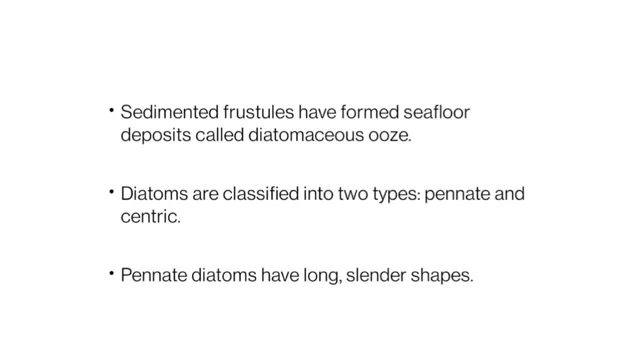 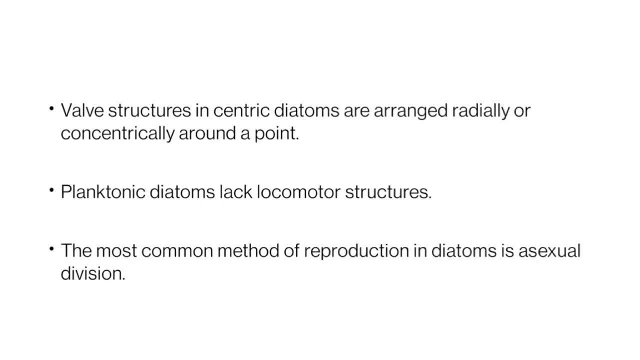 one is the pinnate diatom and the other one is the centric diatom. the pinnate diatom is: these diatoms have an elongated shape and in centric diatoms, the centric diatoms have valves that are arranged radially or concentrically around a point. 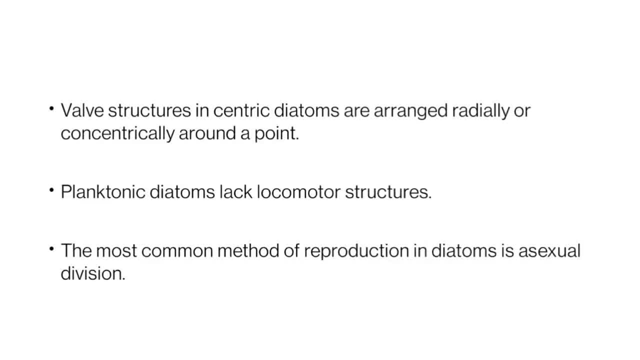 and the most common method of reproduction in diatom is asexual division and in diatoms the method of reproduction is asexual division. and sexual division is also present when diatoms are formed and the height of the diaphragm, or when diatom reaches a certain critical minimal size, it 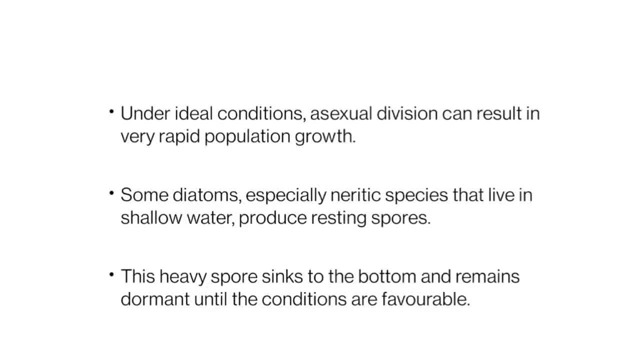 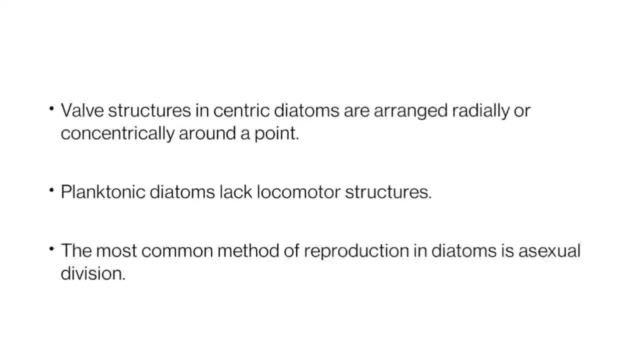 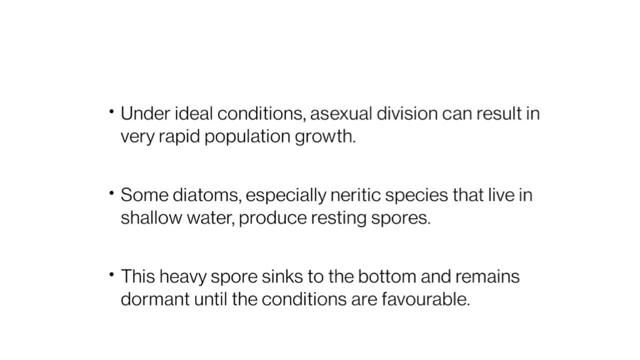 undergo sexual reproduction also, and this because of this asexual reproduction and and which results in the very rapid population growth under optimal uh conditions, And some diatoms, especially neurotic species that live in shallow water, produce the rusting spores, And these heavy spores actually sink into the bottom and remain dormant until favorable situations. 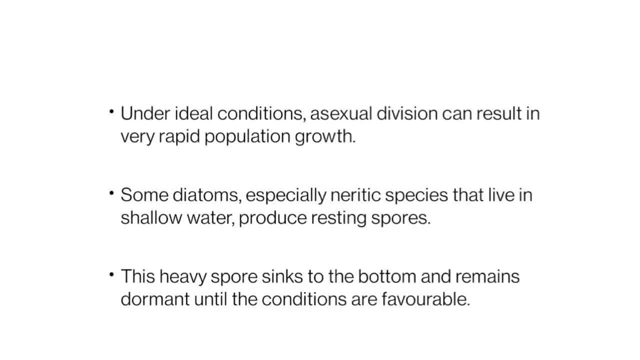 And during unfavorable condition, these diatoms produce rusting spores And when a favorable condition came, it will produce normal planktonic cells, Or these spores transformed into a normal planktonic cell. Actually, the study related to these diatoms, the spores and cysts of these diatoms, is a good research topic. 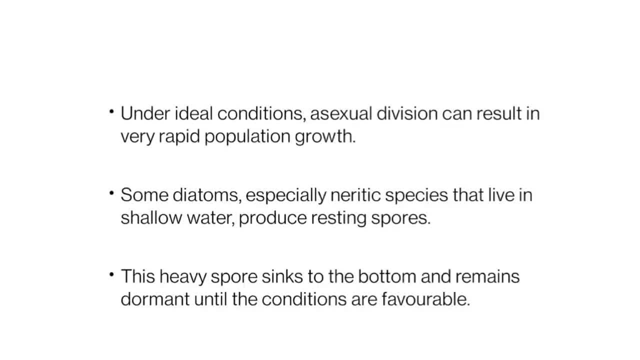 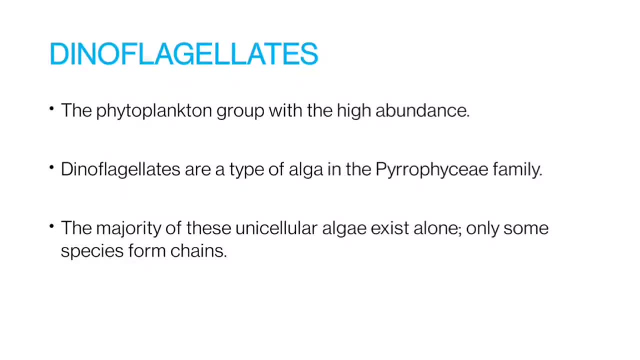 planktonic cell. actually, the study related to these diatom, the spores and assists of this diatom, is a good research topic. next one is dino flagellate, the plankton group with the high abundance and diant teleotherm. dinoflagellates are a type of algae in the pyrophysia family. the majority of these unicellular 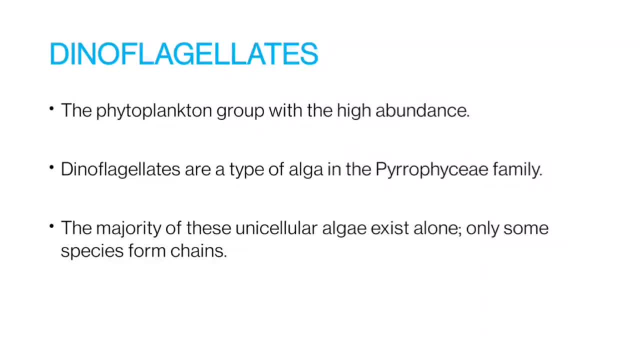 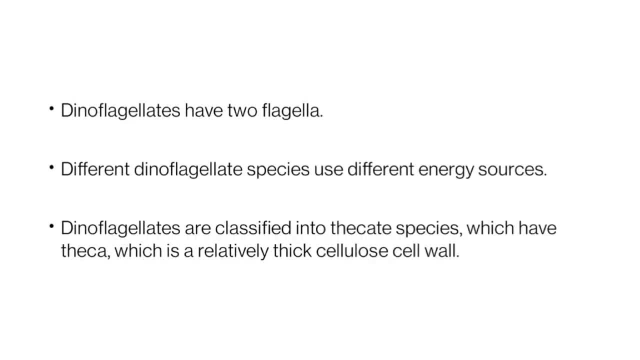 algae exist alone. only some species form chains. dinoflagellates have two flagella, and different dinoflagellate species use different energy sources. so some dinoflagellates are strictly autotrophic in nature and they're building organic materials and obtaining all their energy from photosynthesis, and some other species carry a heterotropic. 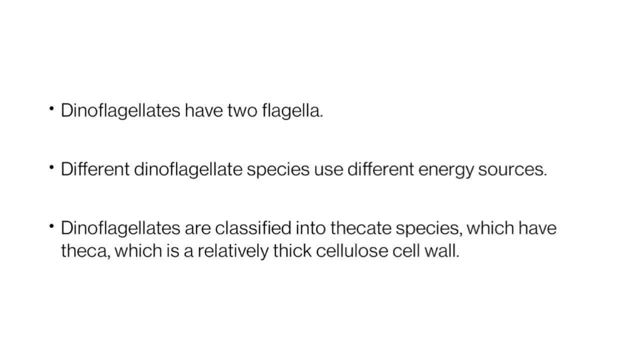 production and actually they meet their energy needs by feeding on phytoplankton or small zooplankton. and indeed 50 percentage of dinoflagellates are strictly heterotropic, and then they actually lack chloroplasts and that are incapable of carrying photos in carrying. 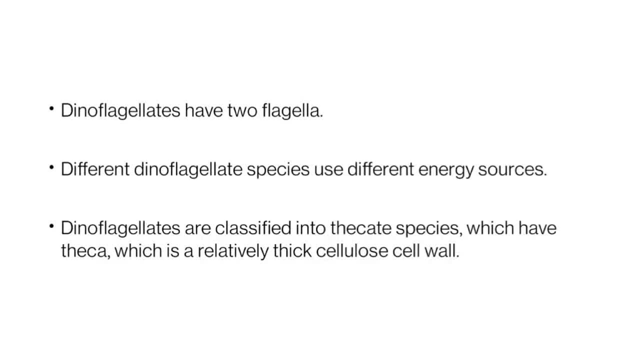 photosynthesis and some dinoflagellates. and some dinoflagellates are mixotropic in nature, that is, they are capable of autotrophic as well as the heterotropic production. the dinoflagellates are classified into ticket species and which have tika, which 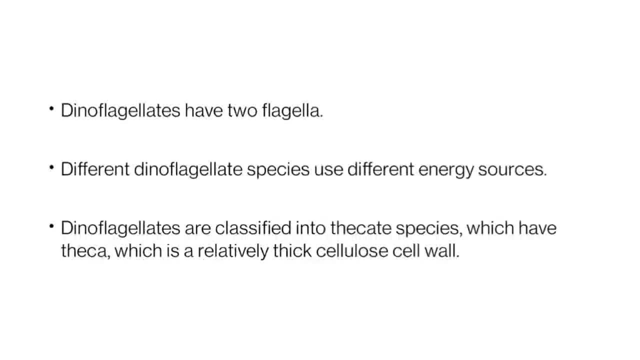 is a relatively thick cellular cell wall, like the the diatoms in the dinoflagellates. they form the thick cellular cell wall called the tika. on the basis of presence and absence of this tika, the dinoflagellates also classified the case. ticket species and naked species are there. 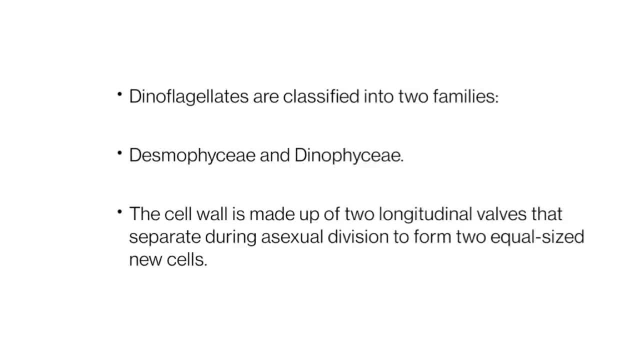 the dinoflagellates are classified into two families: desmophysia and dinophysia. the cell wall is made up of two longitudinal walls that separate during a sexual division to form two equal sized new cells, and sexual. in the method of reproduction in dinoflagellates is 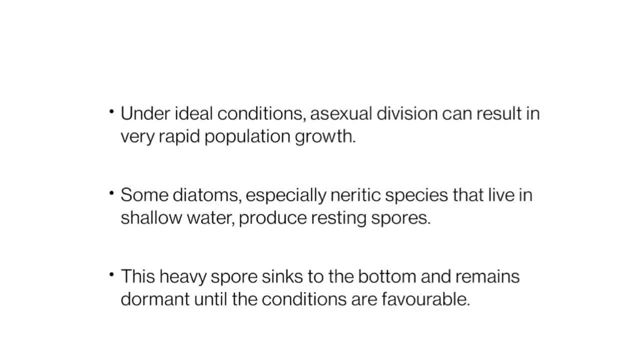 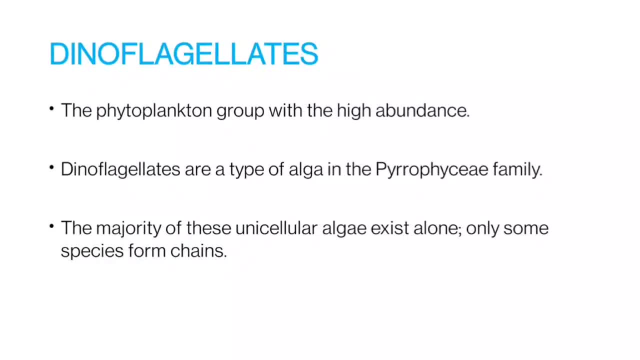 Next one is dinoflagellate. Dinoflagellates are the plankton group with the high abundance, And dinoflagellates are a type of algae in the pyrophysia family. The majority of these unicellular algae exist alone. Only some species form chains. 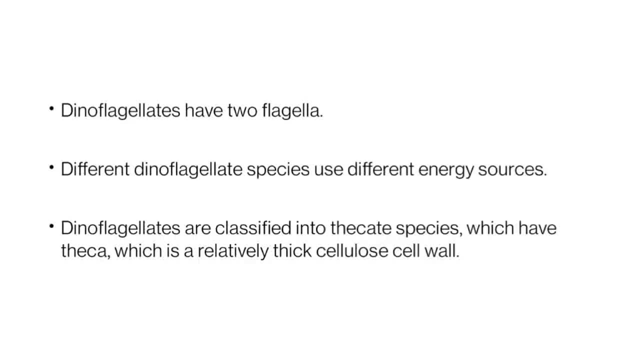 Dinoflagellates have a high abundance of algae. Dinoflagellates have a high abundance of algae. They have two flagella, And different dinoflagellate species use different energy sources. Some dinoflagellates are strictly autotrophic in nature. 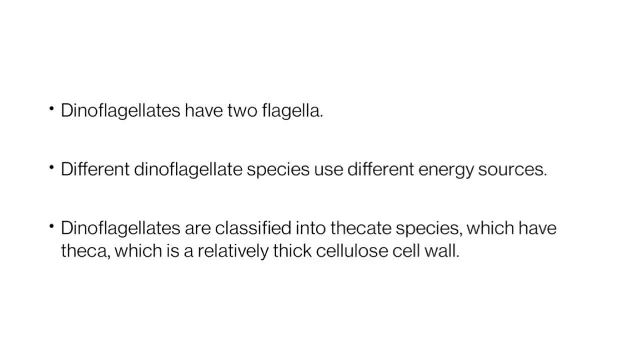 And they are building organic materials and obtaining all their energy from photosynthesis. And some other species carry a heterotropic production And actually they meet their energy needs by feeding. And some other species carry a heterotropic production And they are feeding on phytoplankton or small zooplankton. 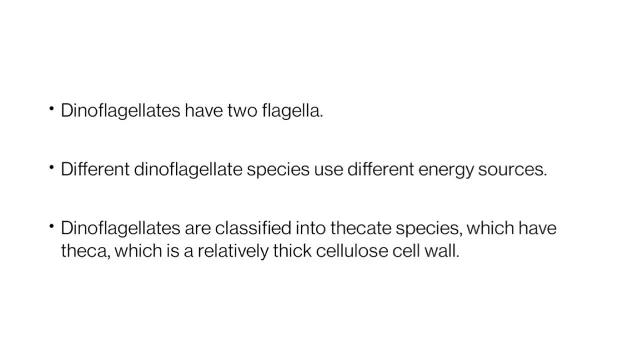 And indeed 50% of dinoflagellates are strictly heterotropic And they actually lack chloroplasts And that are incapable of carrying photosynthesis. And some dinoflagellates are mixotropic in nature, That is, they are capable of autotropic as well as heterotropic production. 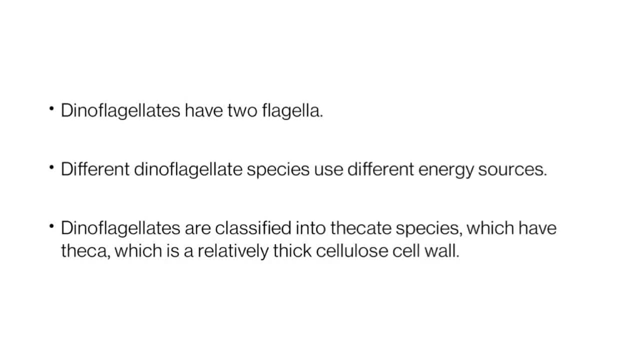 The dinoflagellates are classified into the ecate species And which have theca, Which is a relatively thick cellulose cell wall. Like the prostules in the diatoms In the dinoflagellates, they form the thick cellulose cell wall called the teca. 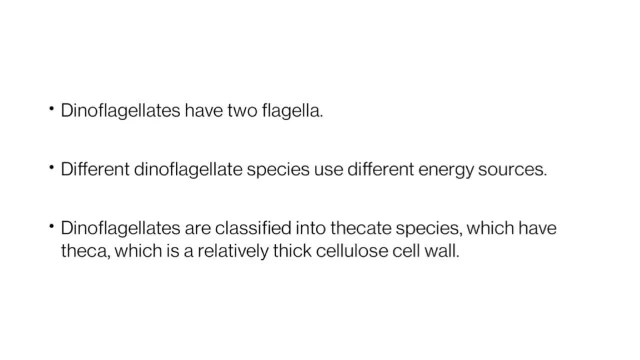 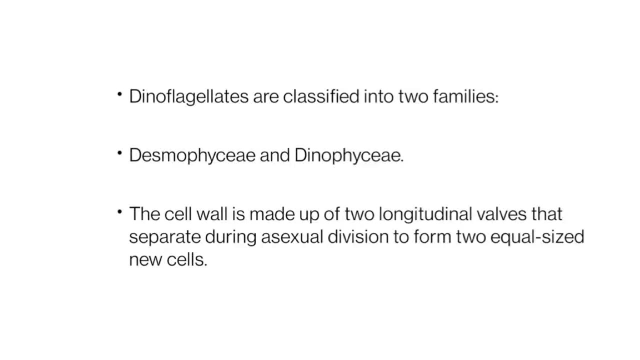 On the basis of presence and absence of this teca. the dinoflagellates, also classified Decade species and naked species are there. the dinoflagellates are classified into two families: desmophysia and dinophysia. the cell wall is made up of two longitudinal walls that separate during asexual division. 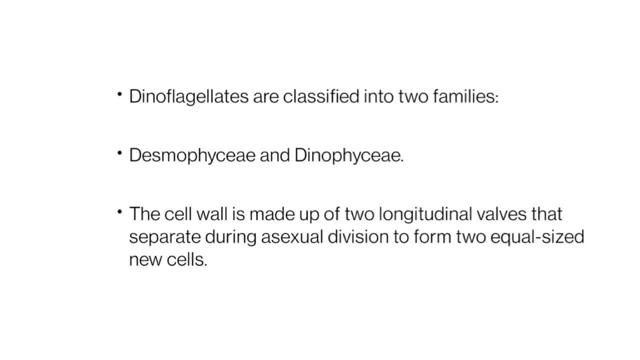 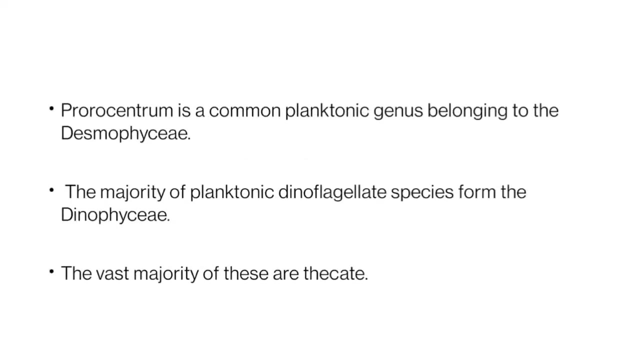 to form two equal sized new cells and sexual. in the method of reproduction dinoflagellates is sexual reproduction- sorry, asexual reproduction and also sexual reproduction also occur in at least some species of dinoflagellates. proro syndrome is a common planktonic genus belonging. 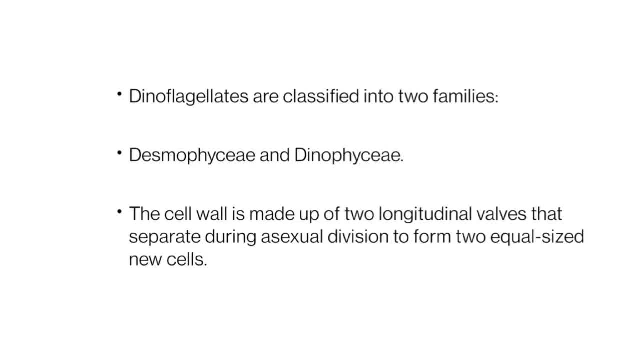 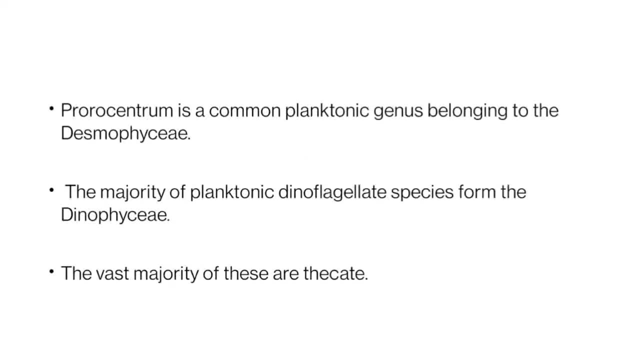 sexual reproduction. sorry, asexual reproduction and also sexual reproduction also occur in at least some species of dinoflagellates. proro syndrome is a common planktonic genus belonging to the desmophysia and the majority of planktonic dynoph. nenhuma species from the dinofici. a vast majority of these are ticket species. 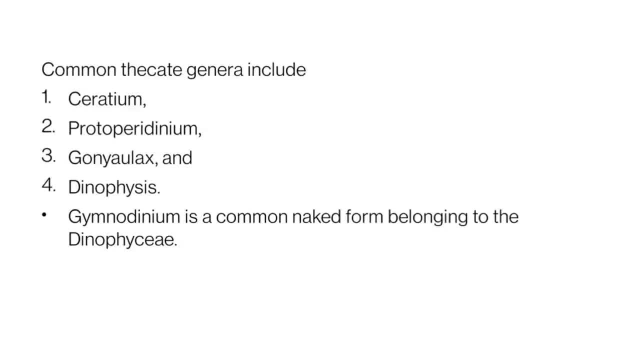 and these are some of the example of these ticket species: serratim prottoperidinium coniolax, and the dinophysis and the gymnotinium is a common ne 헤d form belonging to the yn. зависia. these are the 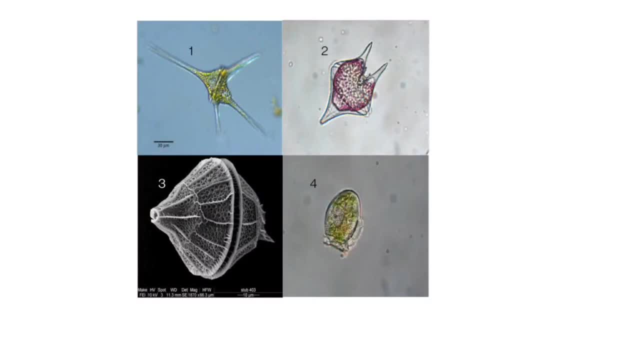 images of species of stella etấn, woodlanded Creek Islandena, between 1697-1979 s caposcillinum and a Cortes fossilised esle ic dating from 1796, for precisely the middle ages. but such first one is serratia, second one protopyridinium, third one goniolax and the fourth one is dinoficy. 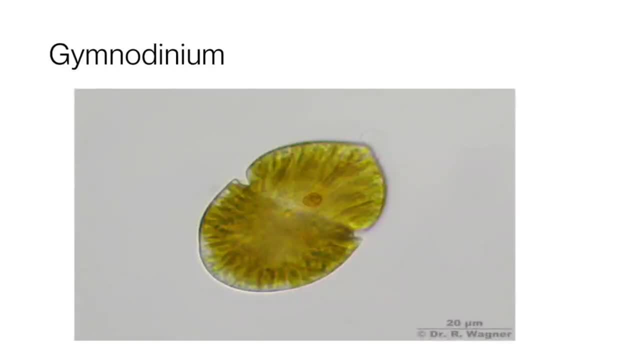 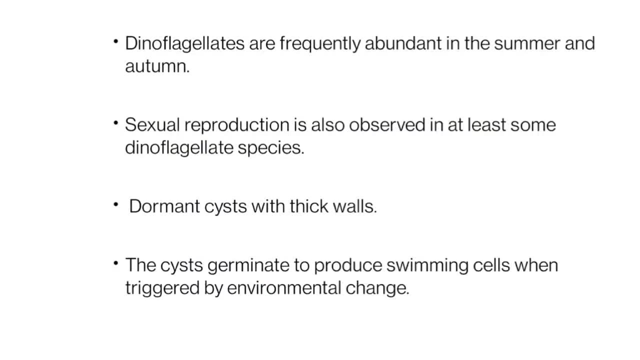 and this is gymnodinium. the dinoflagellates are frequently abundant in the summer and autumn season and sexual reproduction is also observed in at least some dinoflagellate species and i already mentioned, and here also, like the diatoms, they form dormant cysts with the thick walls. this is germinate. 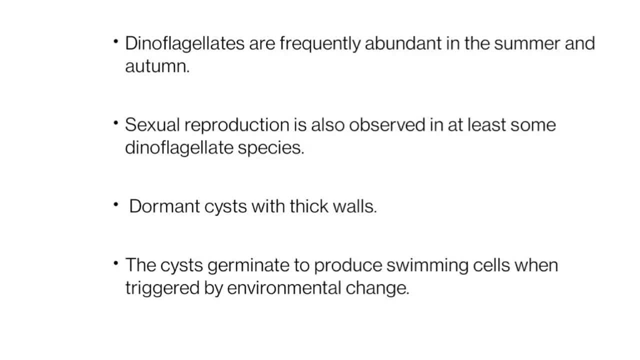 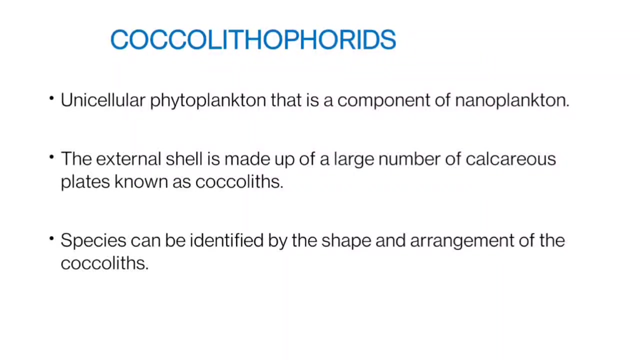 to produce swimming cells. when triggered by the environmental changes and under favorable environmental factors in the environment, they are transformed into planktonic cells like that i mentioned in about the diatoms. next one is the coccolithophores and they are the unicellular phytoplankton that is a component uh- unicellular phytoplankton that. 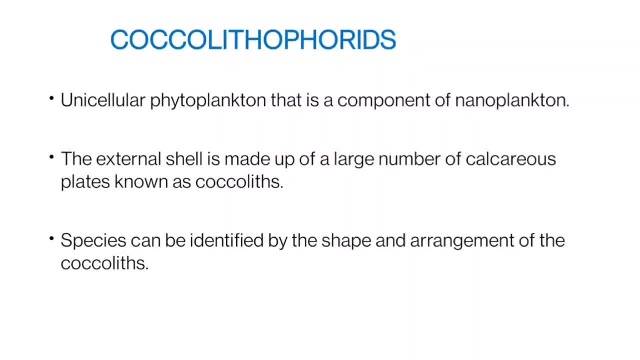 is a component of the nanoplankton uh. nanoplankton, which is they are smaller than 20 micrometer. the external shell of this coccolithophore is made up of a large number of calcareous plates, known as the coccolithophore in diatoms uh. 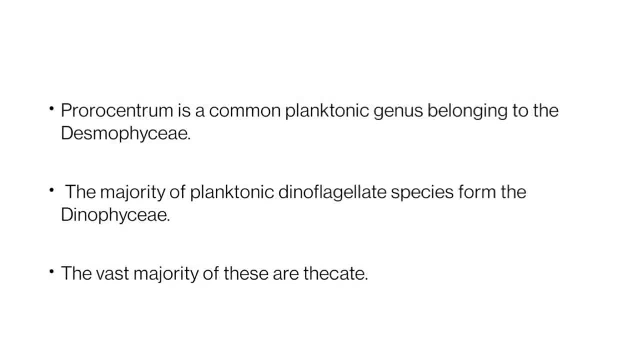 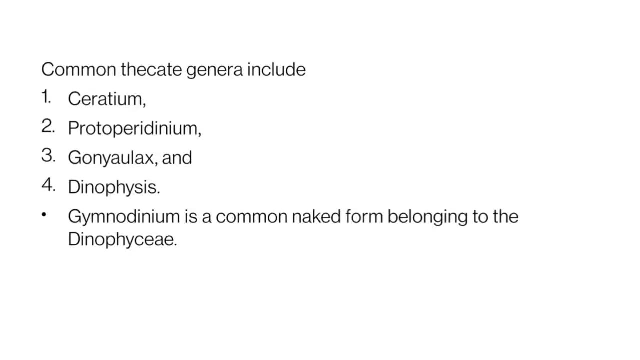 to the desmophysia, and the majority of planktonic dinoflagellate species form the dinophysia. a vast majority of these are thecate species, and these are some of the example of these thecate species: serratium, protoperidinium, corneolax and the dinophysis. 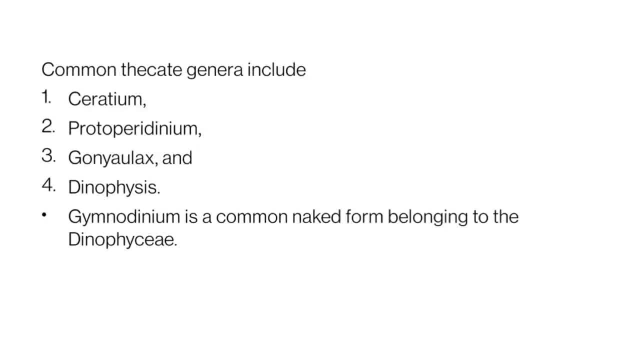 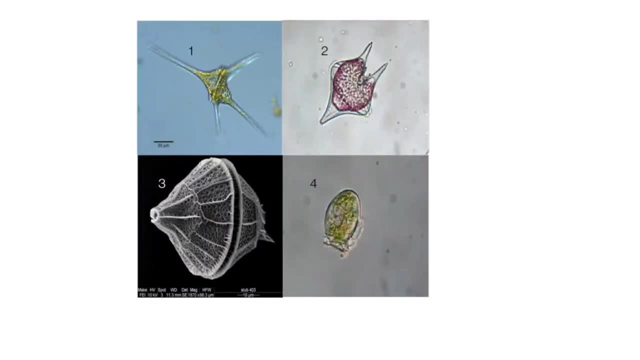 and the gymnosophia. within is a common naked phone belonging to the dinophysia. these are the images of species: first one is serratium, second one in protoperidinium, third one cornealax, and the fourth one is diagonals, and this is gymnosophia. 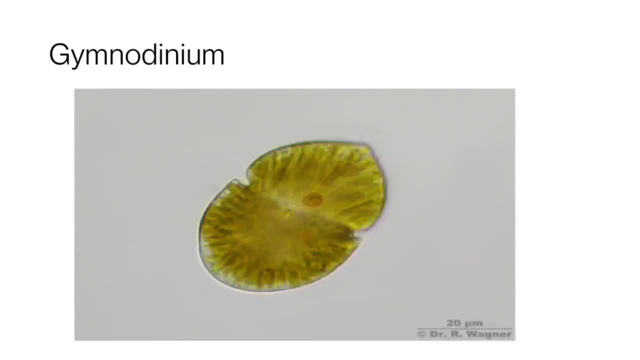 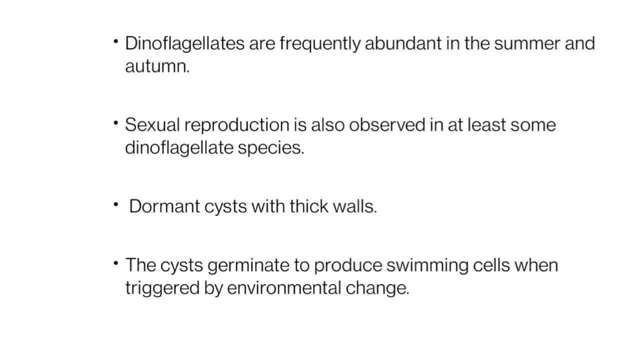 the dinoflagellates are frequently abundant in hacer. how much is they? children, children from which didORTAC-as, my com갈, affecting what 지나 flagent might happen in her mo文公 μ. Foods for your body. flagellates are frequently abundant in the summer and autumn season and sexual reproduction. 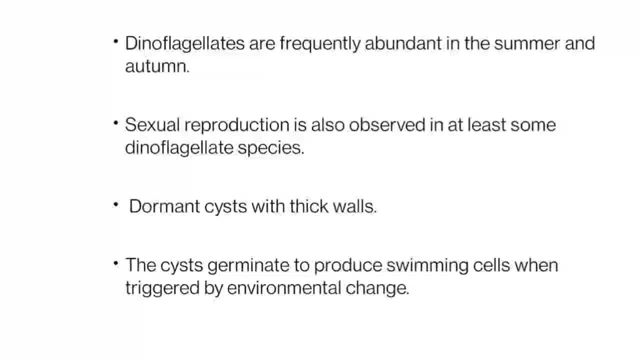 is also observed in at least some dinoflagellate species and i already mentioned, and here also, like the diatoms, they form dormant cysts with the thick walls. the cysts germinate to produce swimming cells when triggered by the environmental changes and under favorable environmental. 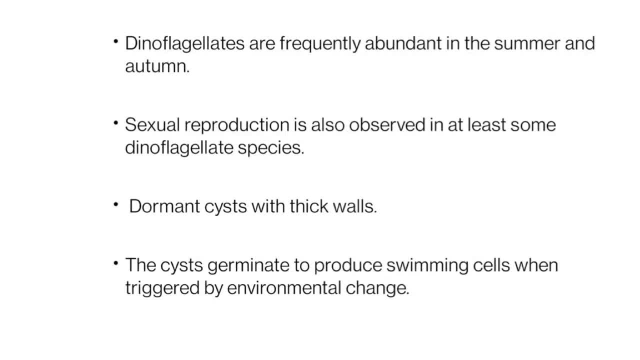 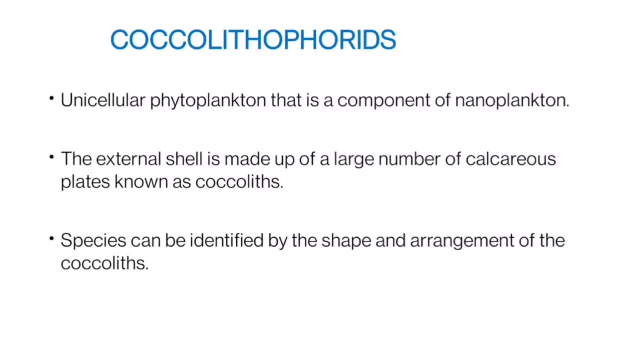 factors in the environment, they are transformed into planktonic cells like that i mentioned in about the diatoms. next one is the coccolithophores and they are the unicellular phytoplankton that is a component- unicellular phytoplankton that is a component of the diatoms and they are the unicellular phytoplankton that is a component. 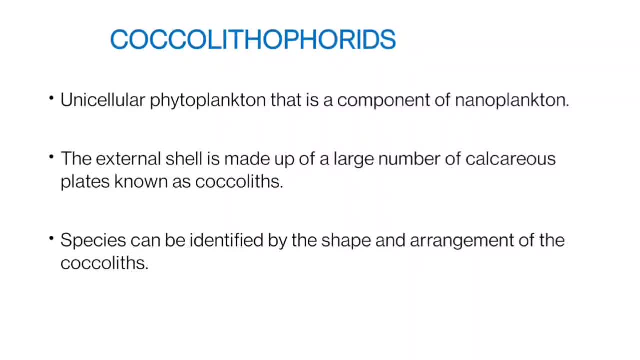 the nanoplankton, uh nanoplankton, which is they are smaller than 20 micrometer. the external shell of this cocolithophore is made up of a large number of calcareous plates, known as the cocolithophore in diatoms, their external shell is actually made up of uh silica, and here in cocolithophore, 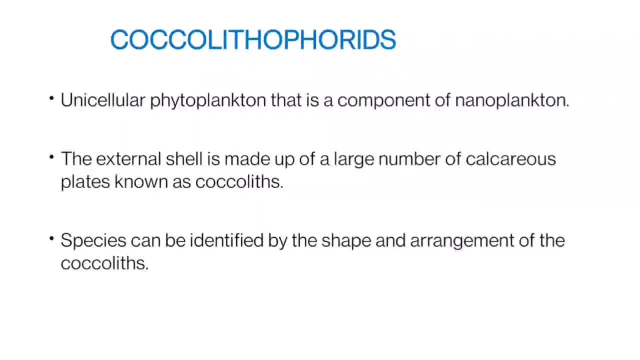 their external shell is actually made up of uh, silica, and here in coccolithophore, the cell is made up of. oh sorry, the external shell is made up of calcareous plates in uh in. in the case of diatoms, they form siliceous, and here this coccolithophore. 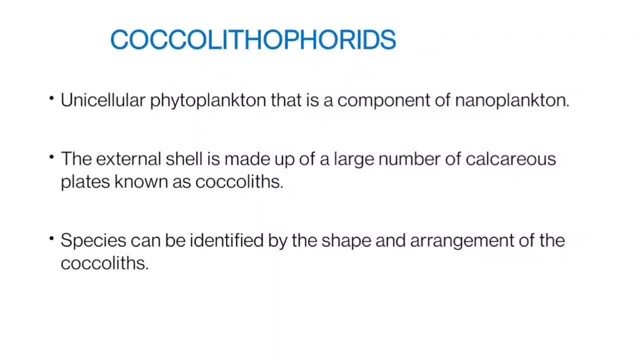 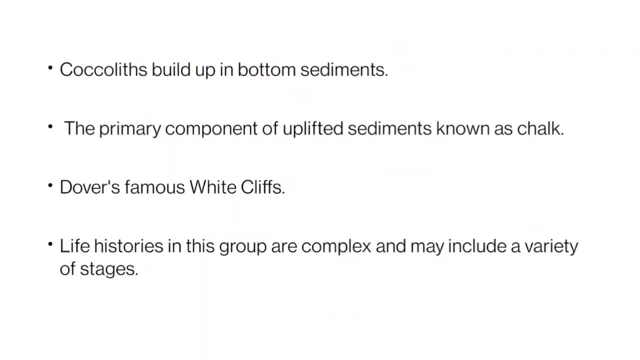 is a death, and death of this coccolithophore results in the formation of calcareous ooze, and these species can be identified by the shape and arrangement of the coccolithophores. coccolithophores build up in bottom sediment and the primary component of the uplifted sediment. 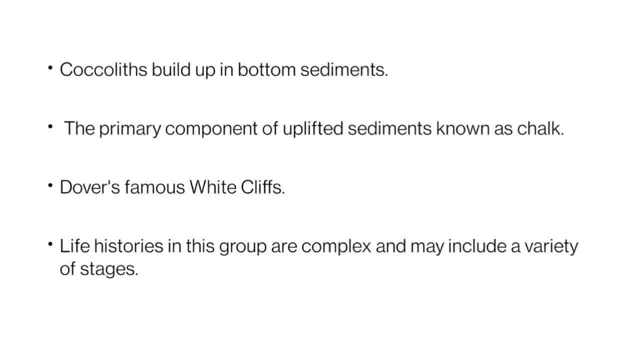 known as chalk, and one example of the the famous dowell's white cliff or the white cliff of dover. in fact, this white cliff of dover contain uh fossilized coccolithophores and the coccolithophore fossilized remaining of this coccolithophores. life histories in this group are complex and 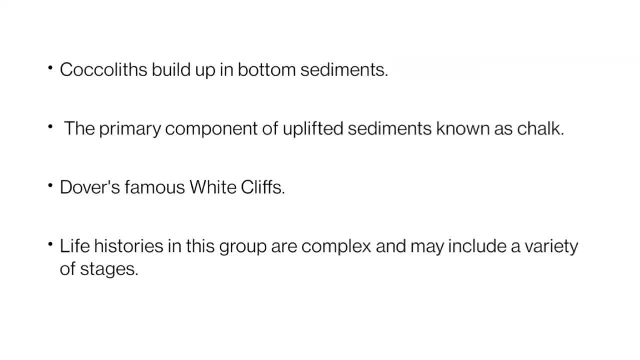 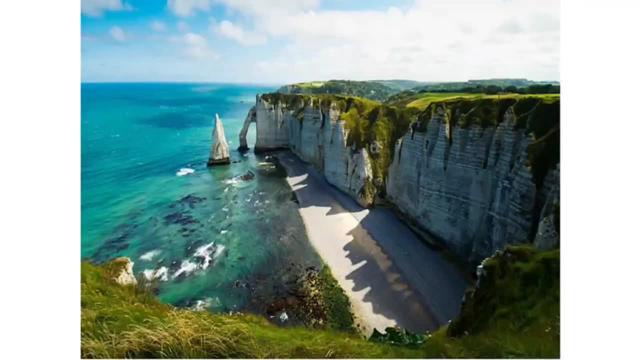 may include a variety of stages, and this is the white cliff of dover in england, and actually they are made up of uh this. i already mentioned that fossilized coccolithophores are present and actually, after the death of this uh coccolithophore, they gradually sink to the 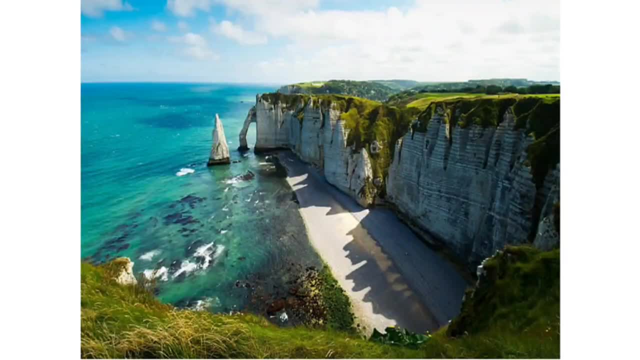 very bottom and lay there on the sea floor, and then over a hundred of uh died and stocked up and, as a result, due to the intense pressure of the uh sea water and the calcium carbonate containing the coccolithophore compress and uh, form uh. this, uh like structure like this and the 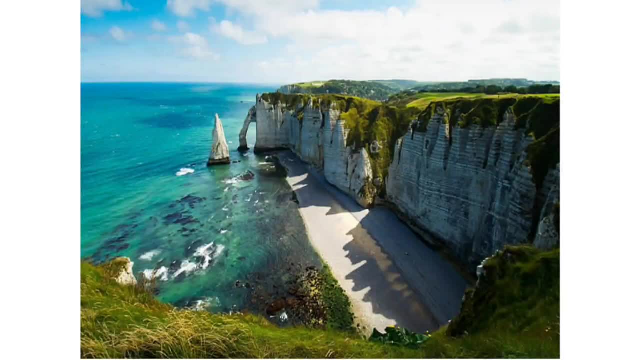 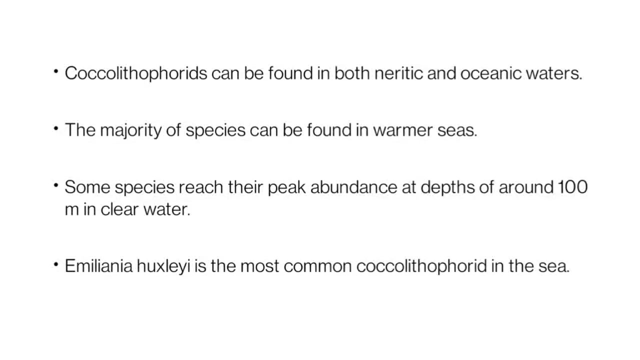 coccolithophores are found in both the neuritic and oceanic waters. due to the plan uh this plated tectonic activities uh, this particular structure uh was under the ocean and it is uplifted or raised up to the up and, as a result, this white cliff of tower formed. coccolithophores can be found in both. 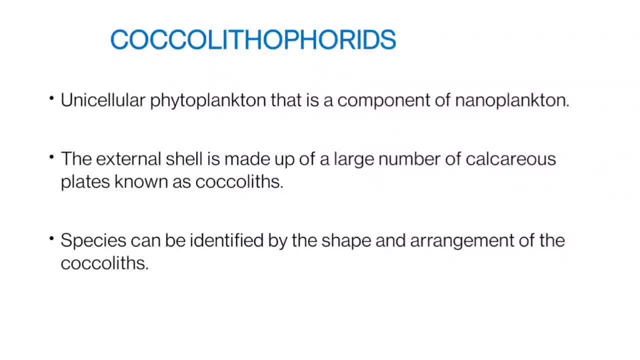 the cell is made up of- oh sorry, the external shell is made up of calcareous plates in uh in. in the case of diatoms, they form siliceous, and here this cocolithophore is the death, and death of this cocolithophore results in the formation of calcareous. 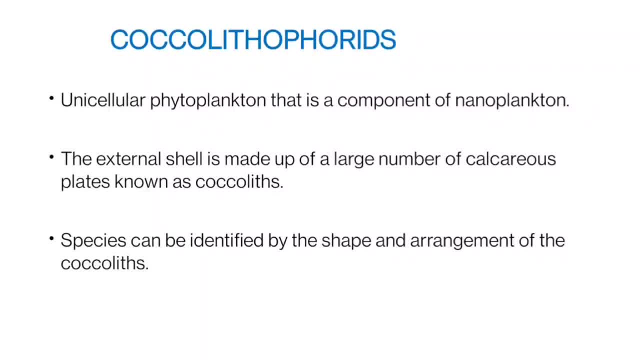 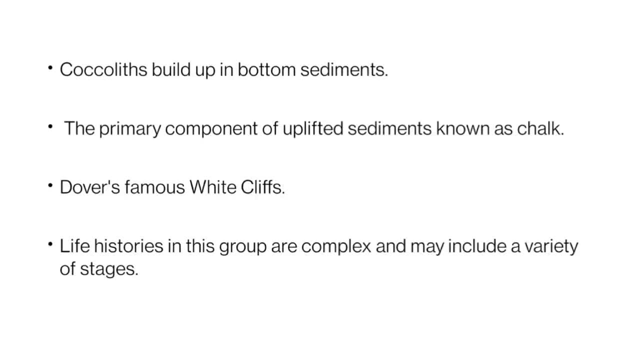 and this species can be identified by the shape and arrangement of the cocoliths. cocoliths build up in bottom sediment and the primary component of the uplifted sediment stoke. and one example of the, the famous dover's white cliff, or the white cliff of dover, in fact. 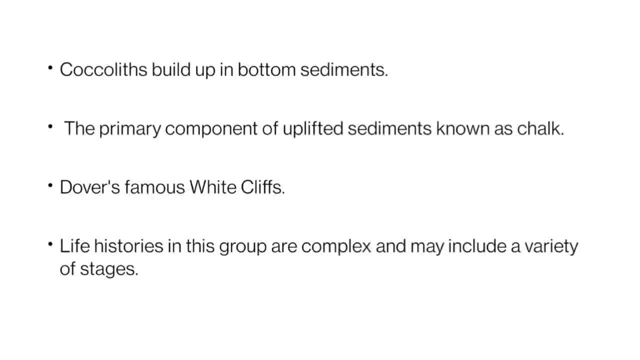 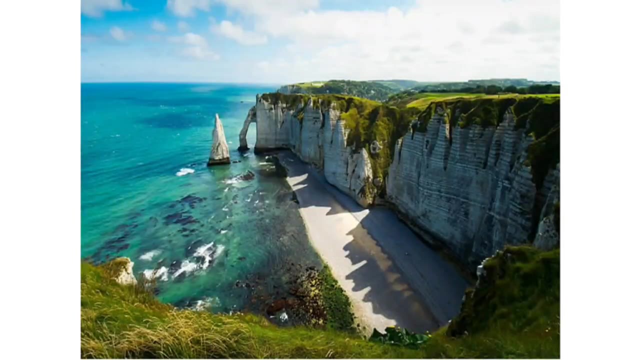 this white cliff of dover contain fossilized remaining of this cocolithophores. life histories in this group are complex and may include a variety of stages, and this is the white cliff of dover in england and actually they are made up of this. i already mentioned that fossilized 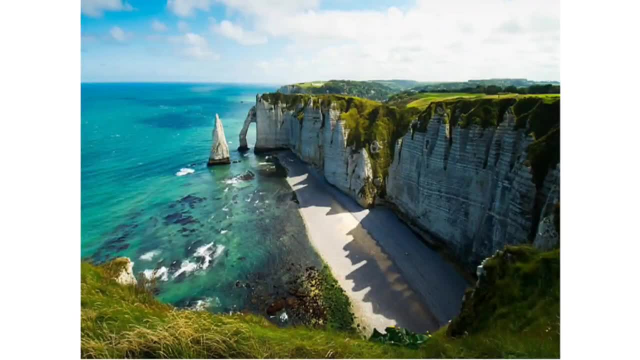 cocolithophores are present. actually, after the death of this uh cocolithophore, they gradually sink to the very bottom and lay there on the sea floor, and then over a hundred of uh died and stocked up and, as a result, due to the intense pressure of the 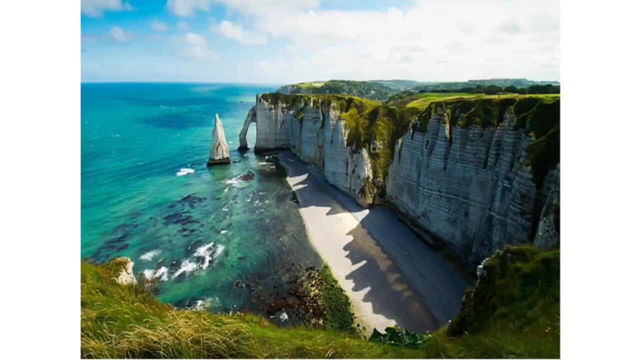 sea water and the calcium carbonate containing the cocolithophore compress and form this like structure like this and due to the plan this plated tectonic activities, this particular structure was under the ocean and it is uplifted or raised up to the up and, as a result, this 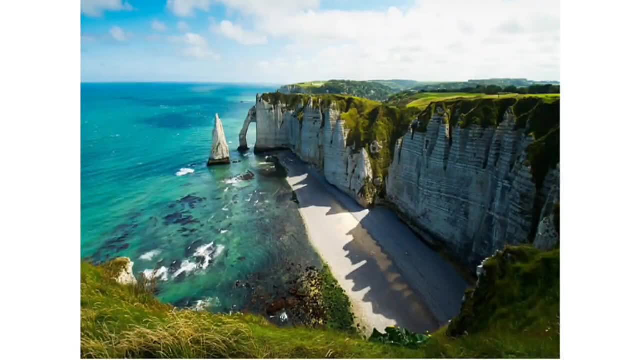 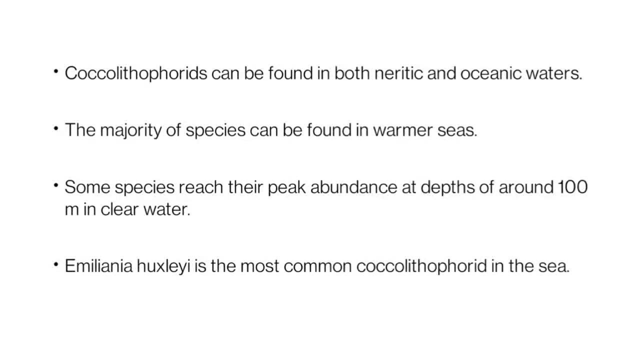 white cliff of tower formed cocolithophores can be found in both the neuritic and oceanic waters. neuritic means uh coastal or a near shore region, near shore environment of, called the co or the coastal waters and the rest of the ocean we are beyond the continental shelf, called the oceanic waters.